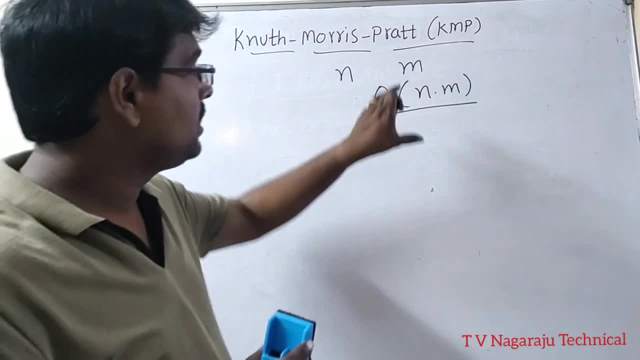 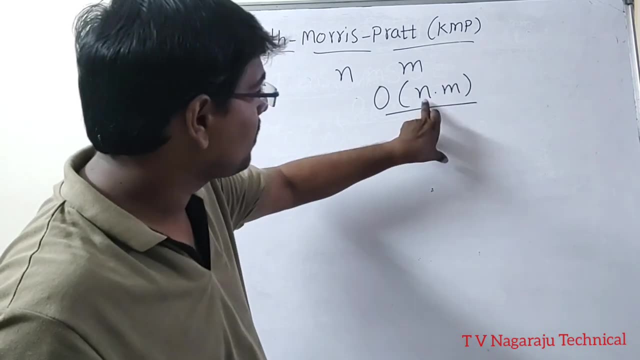 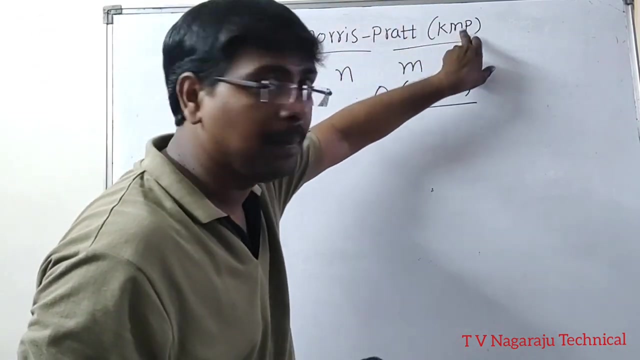 big O of n into m, And this brute force approach also uses backslash Backtracking. Because of this backtracking, only the time complexity of pattern matching increases. Now coming to today's session, KMP algorithm. It generates a time complexity. 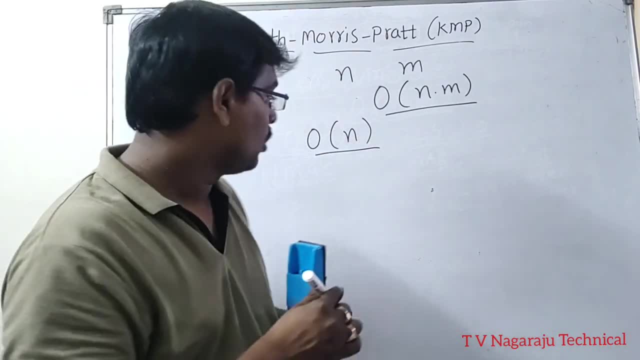 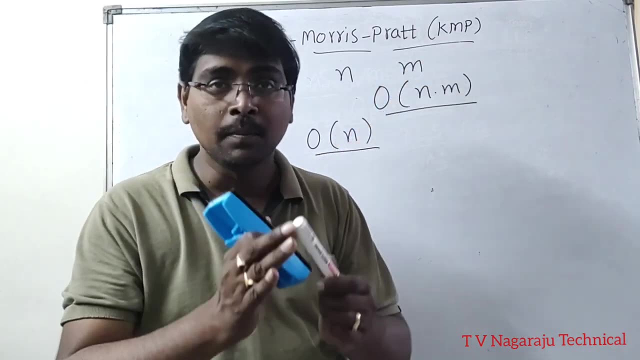 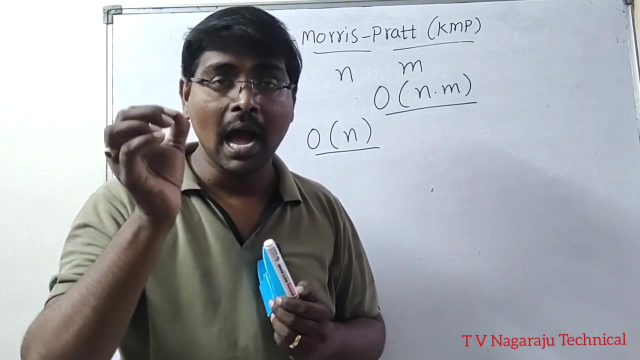 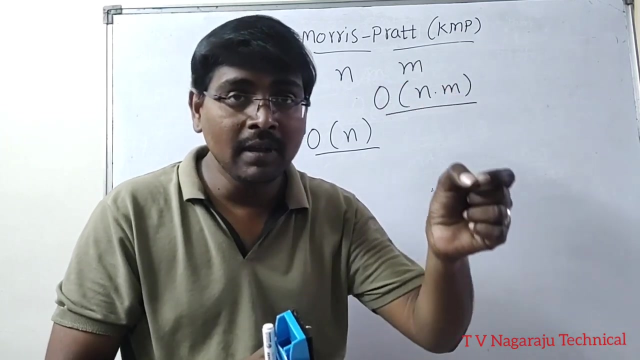 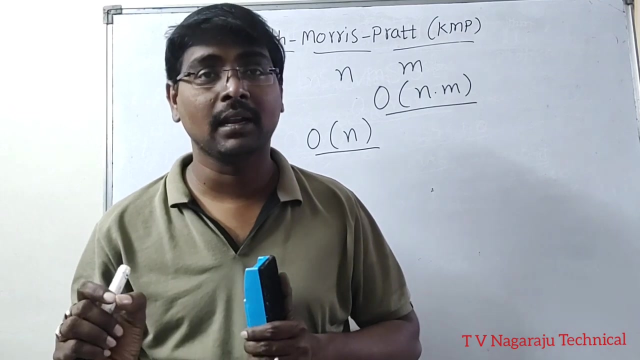 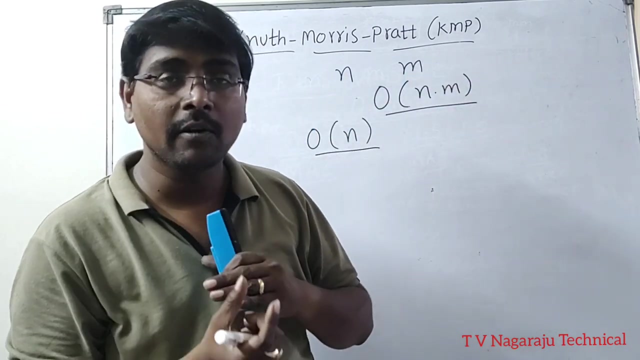 of big O of n. Now, to achieve this time complexity, what the KMP algorithm do, Simply consider n a. So KMP algorithm will determine time state and height of a sheet of paper. Okay, Adding and subtracting time complexity of this pattern. 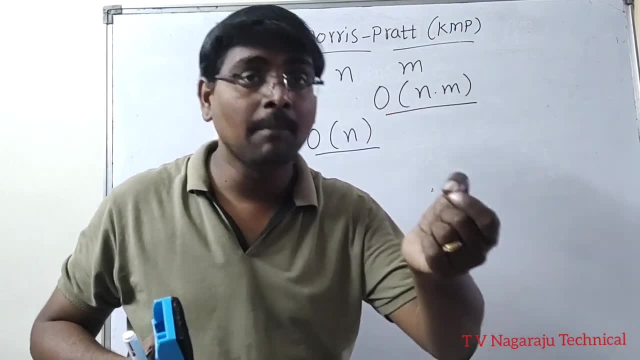 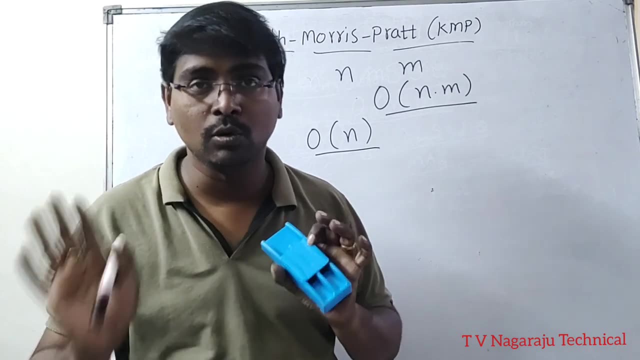 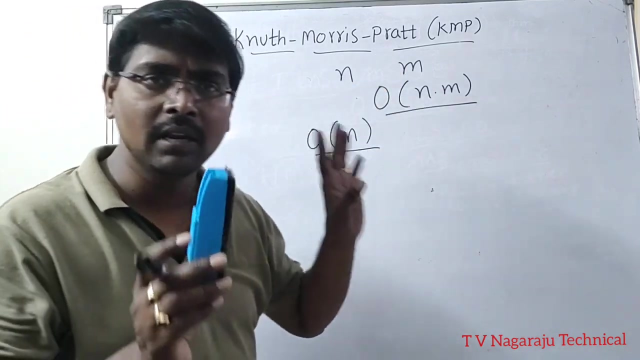 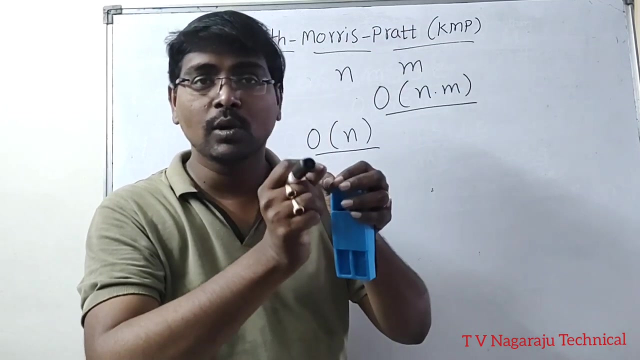 ok, ok, ok. Now해야 攻 18. Now you need to avoid the comparison one more time. That means backtracking is not achieved. Simply how KMS algorithm works. Very, very easy algorithms. How it works. Compare the first two characters of the text with the first two characters of the pattern. 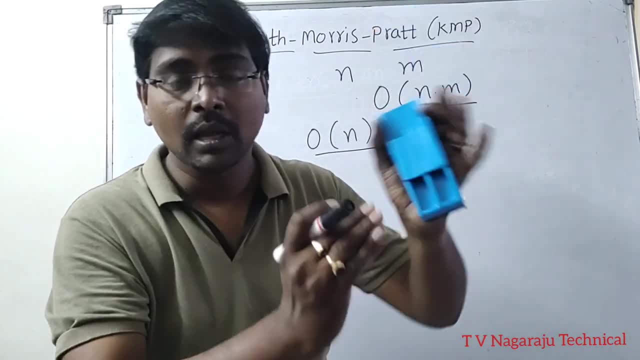 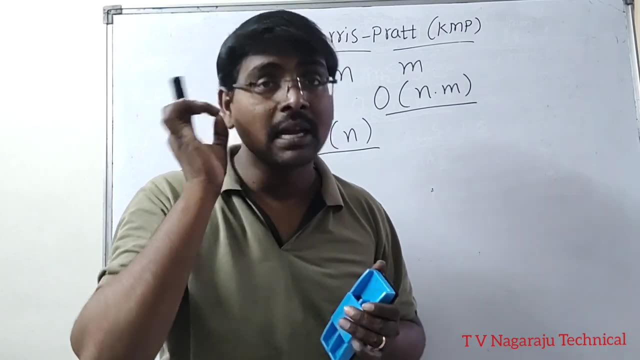 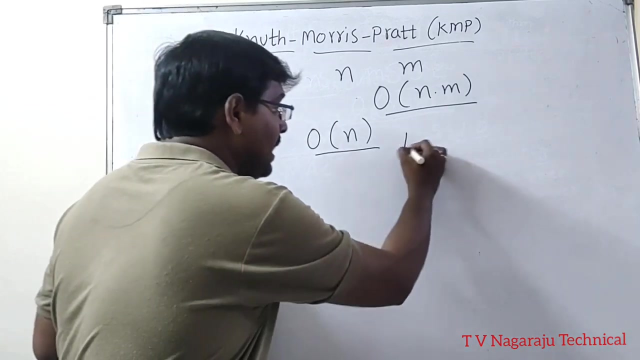 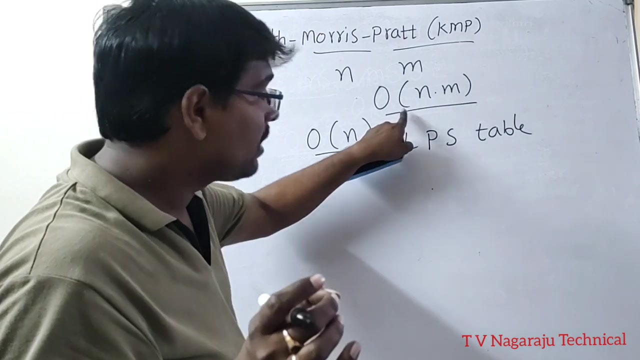 If both are equal, move to second one. If both are equal, move to next one. Whenever there is a failure, that means mismatch occurred, the KMP algorithm uses LPS table Instead of using backtracking. whenever mismatch occurred, the KMP algorithm uses LPS table. 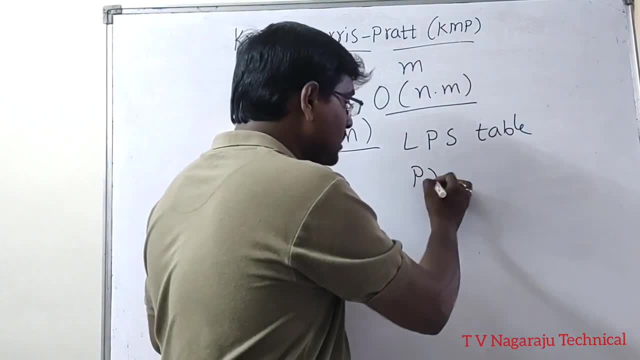 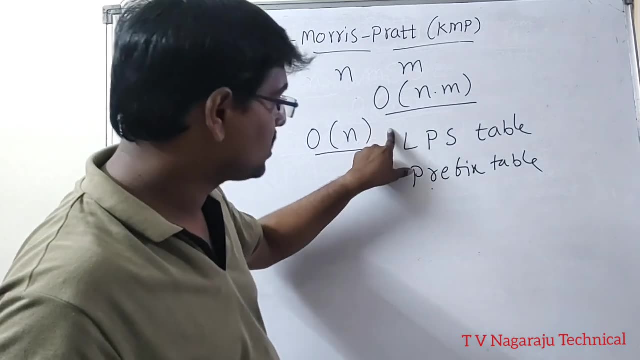 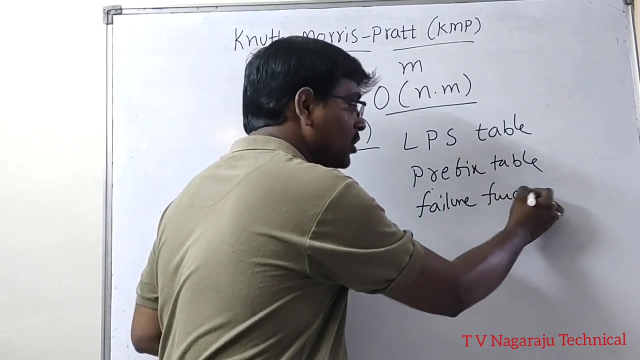 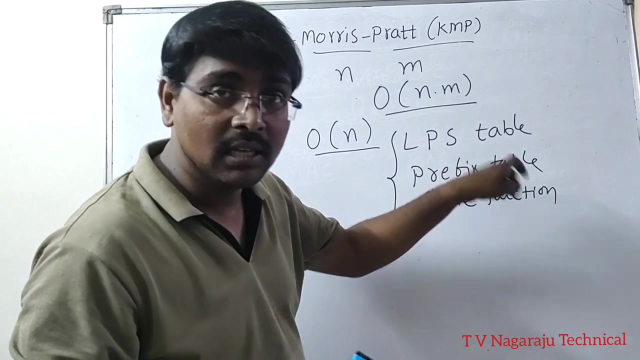 This is also called as prefix table, So a preprocessor table, LPS table, also called as prefix table, also called as failure function. You can call with any name By using this one, only by using this one, only to skip the comparison with the characters. 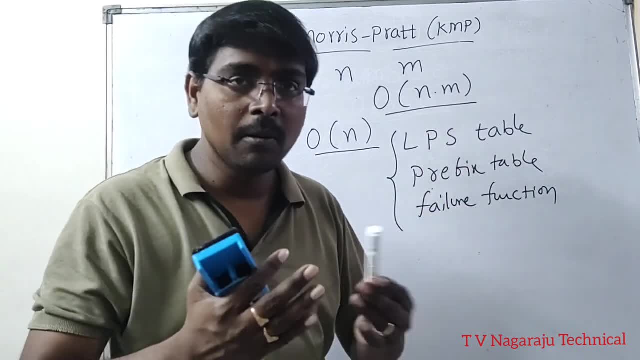 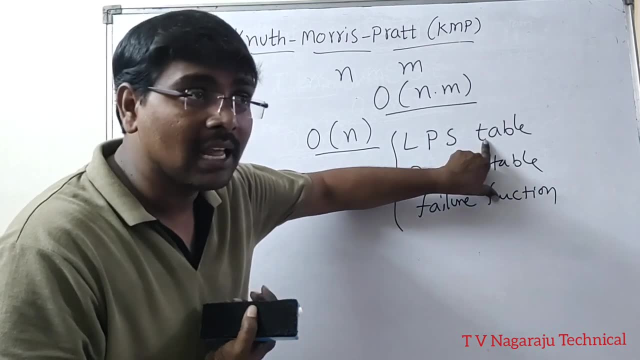 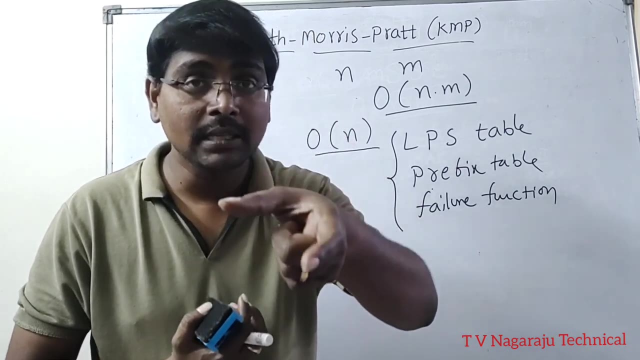 To skip the comparison with the characters. So obviously, what is the first step? Enter into the algorithm. The first step is construct the LPS table. Once the LPS table is constructed, based on the LPS table, apply the KMP algorithm. 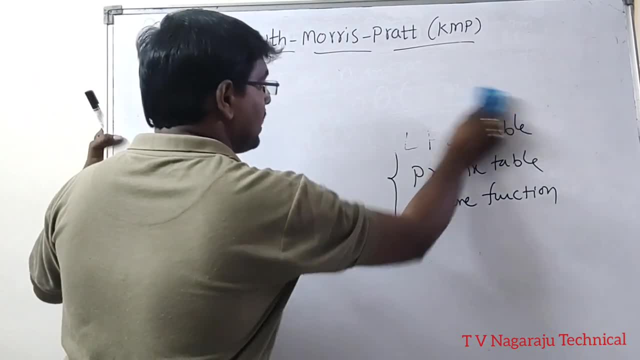 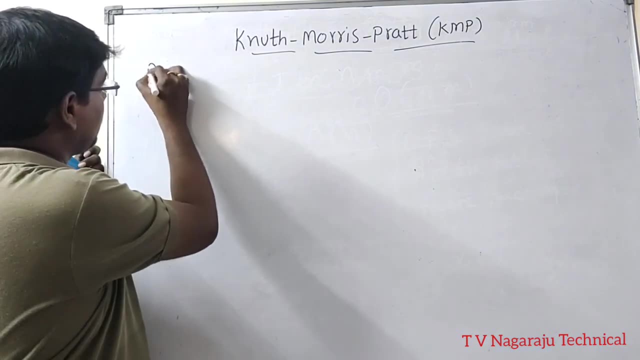 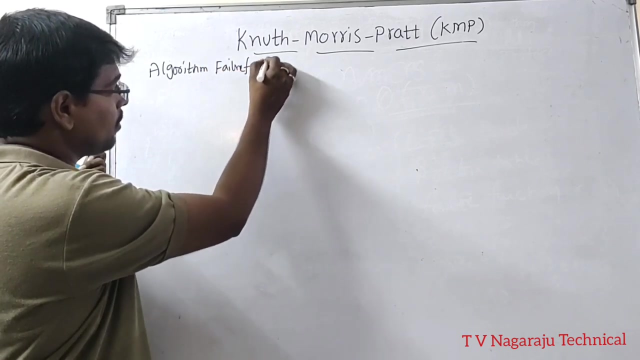 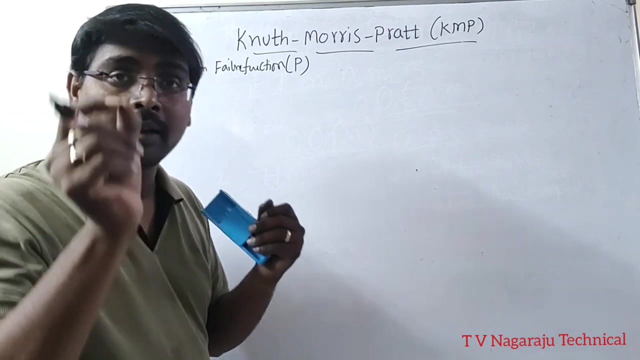 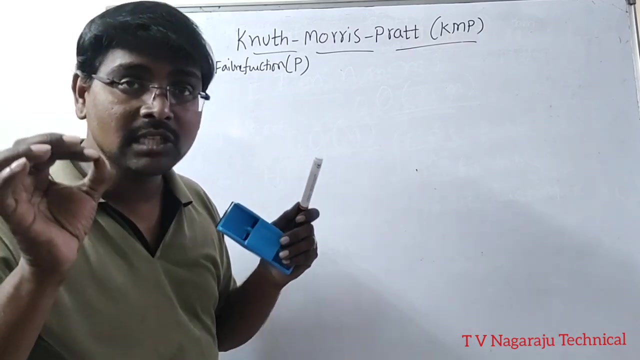 Now I will construct the LPS table and based on this one, I will give you an example also Now. algorithm failure function. You can use any name, not a problem. Failure function of P. What is P? P is the pattern. Remember we are calculating LPS table not for the text. Calculate LPS table for the pattern only. 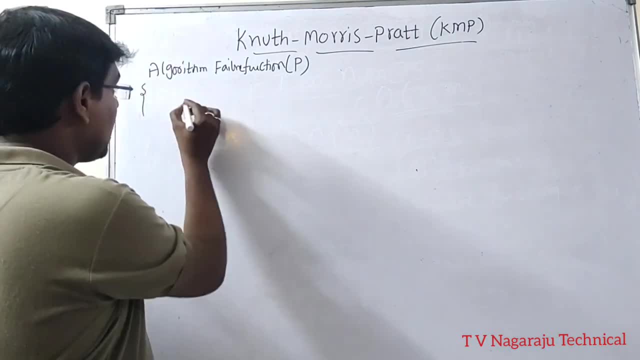 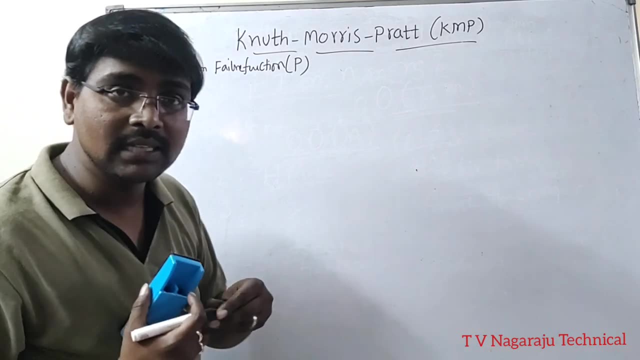 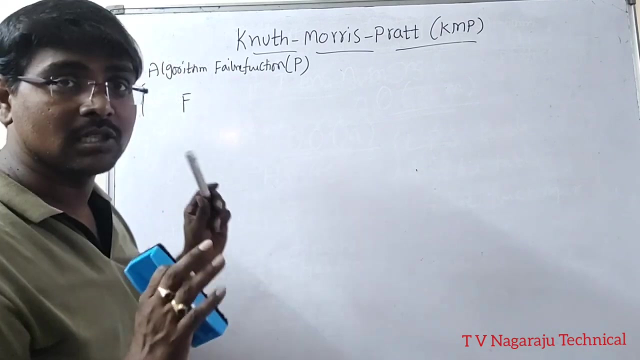 For the pattern, only For the pattern. use one Array F. This is my table. What is the size of table? Size of the pattern. Suppose if pattern consists of some 6 characters, the size of LPS table is 6 characters. 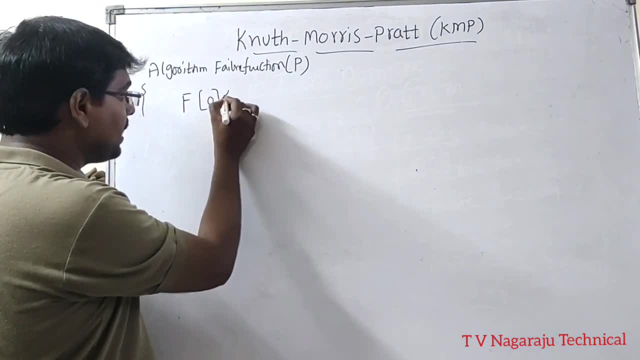 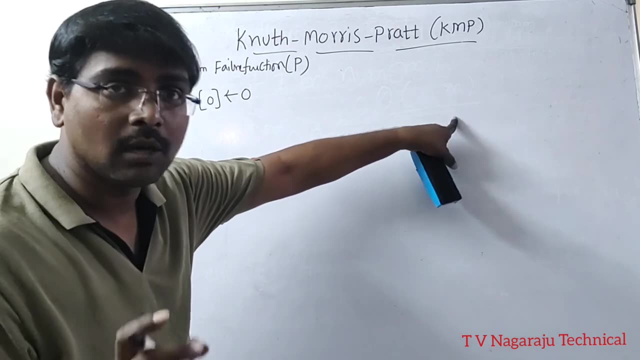 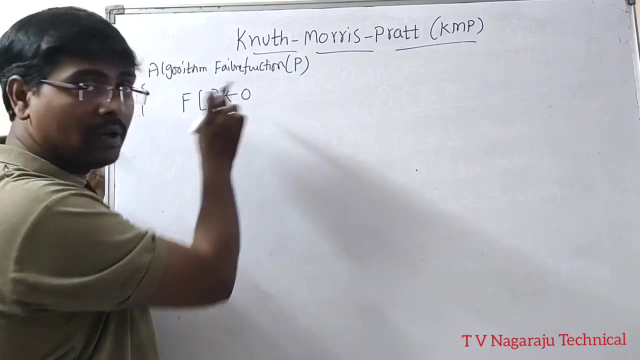 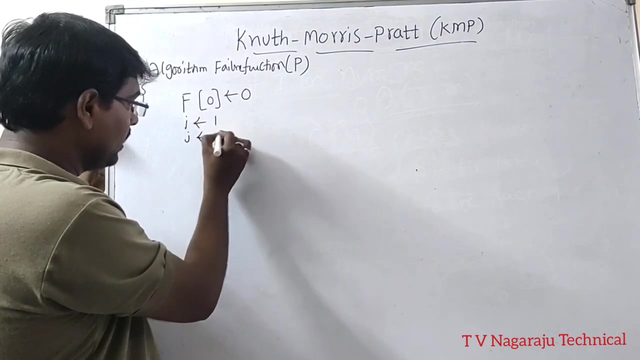 Initially, at 0th position, I placed a value 0. No problem, After completion of example. sorry algorithm. I will give one example. You will understand clearly. At 0th position of the table, I filled a value 0. Now I am taking two values: i is equal to 1, j is equal to 0. 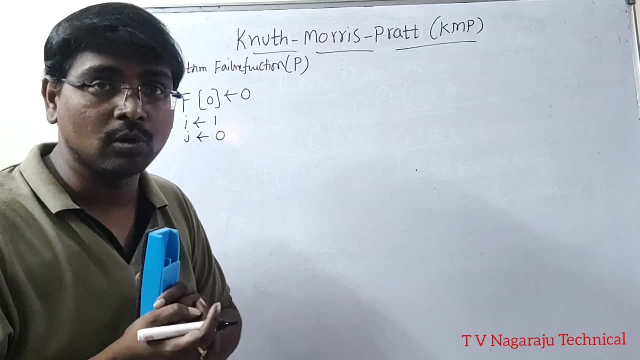 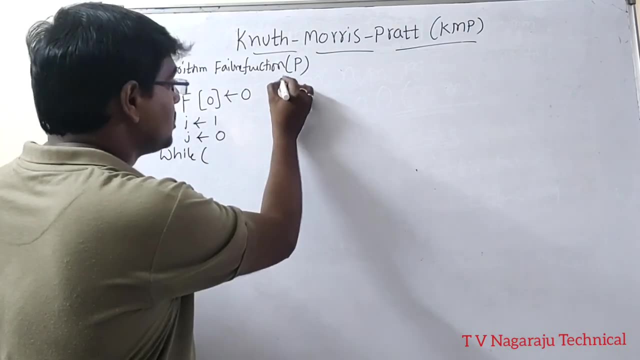 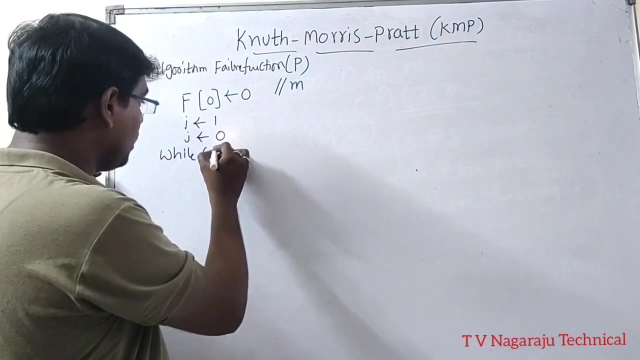 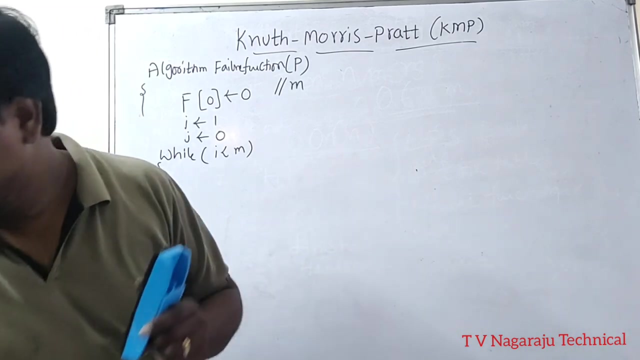 i is equal to 1, j is equal to 0. Now repeat a loop until end of the pattern. Assume m is the length of the pattern. m is the length of the pattern, While i is less than m. while i is less than m, we are repeating the loop. 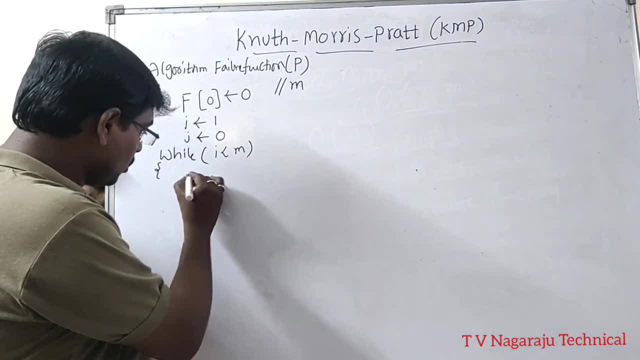 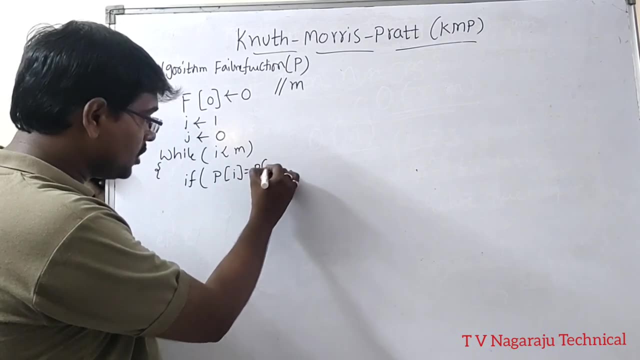 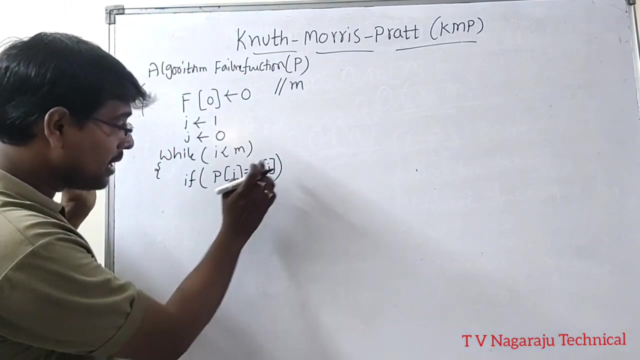 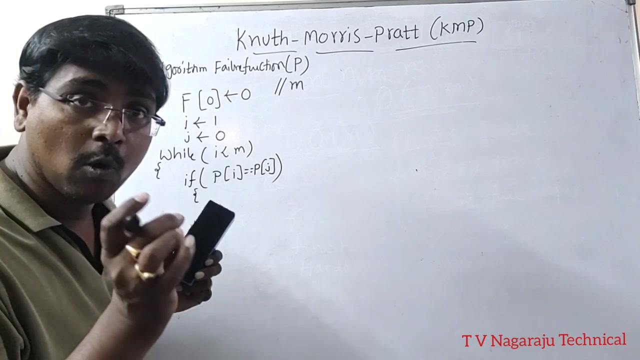 Inside the loop. what we are doing? First, do the comparison. If P of i is equal to P of j, what is the meaning? The first two position character in the pattern is comparison. Suppose if both are equal, then fill the table. 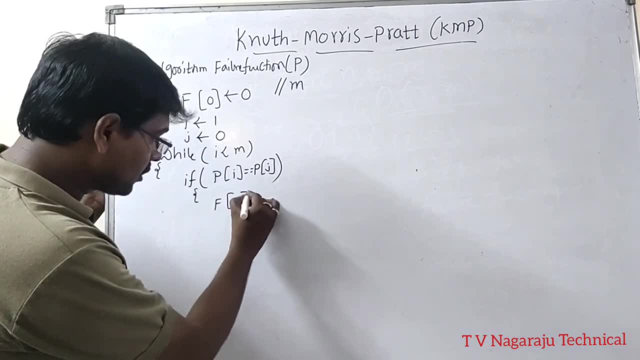 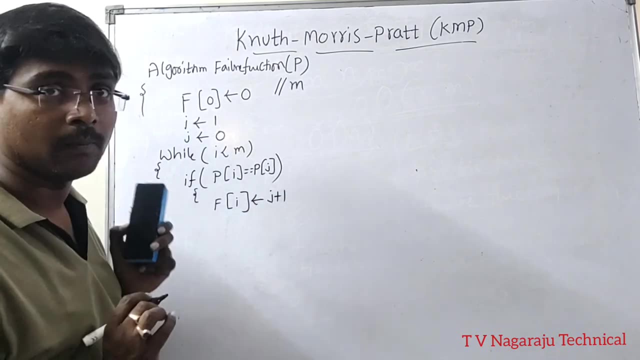 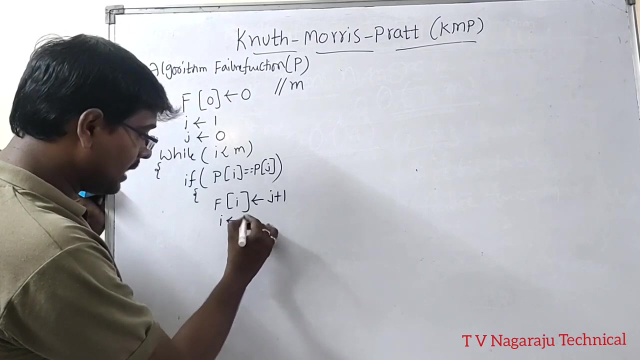 Already, 0th position is completed. Fill the first two position like. first two position means i is equal to 1 with the value of j plus 1.. With the value of j plus 1, after completion, after filling increment, i value by 1.. 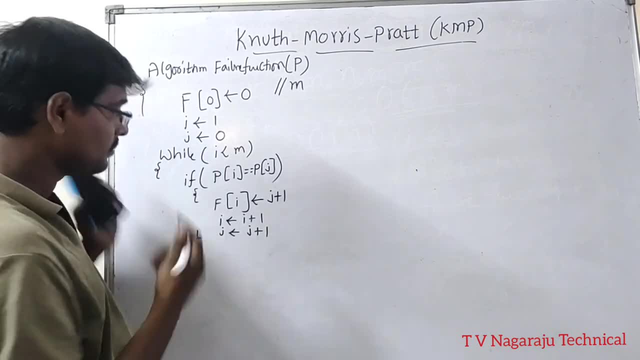 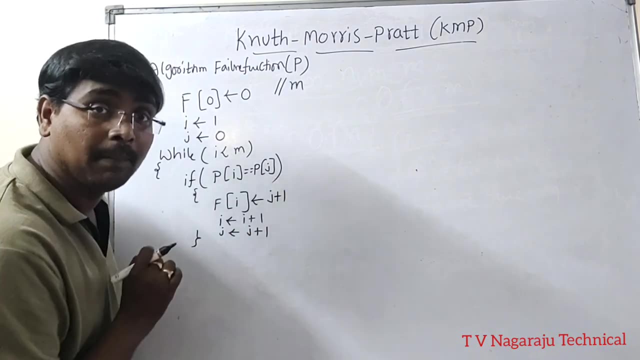 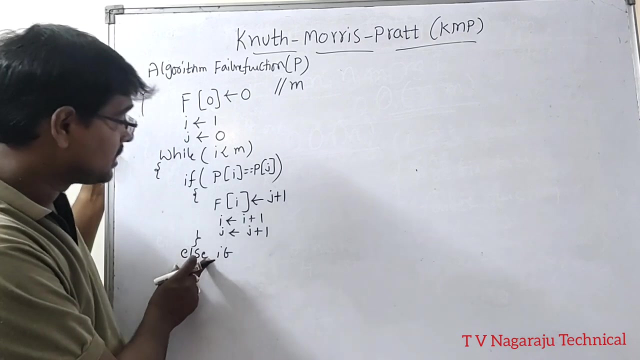 And increment j value by 1.. Increment: i value by 1 and j value by 1.. Suppose: if there is a mismatch, if there is a mismatch, else, if We are coming to, if else, in a sense both are not equal. 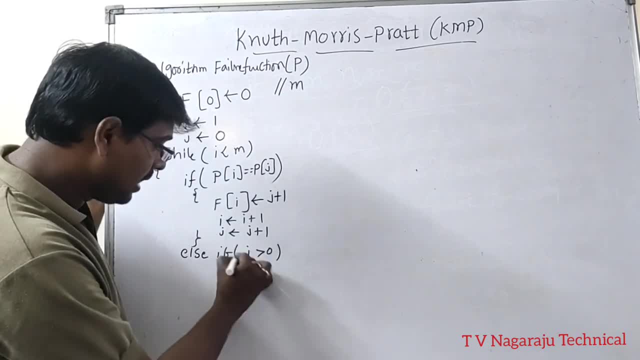 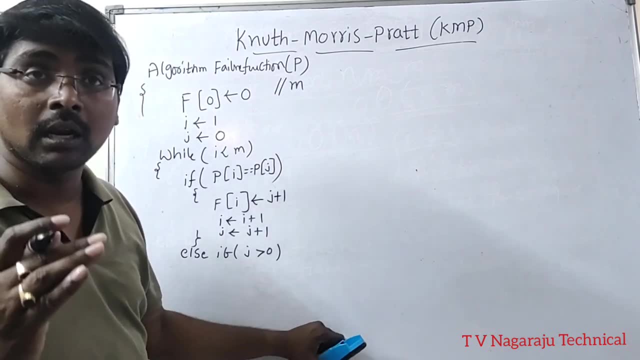 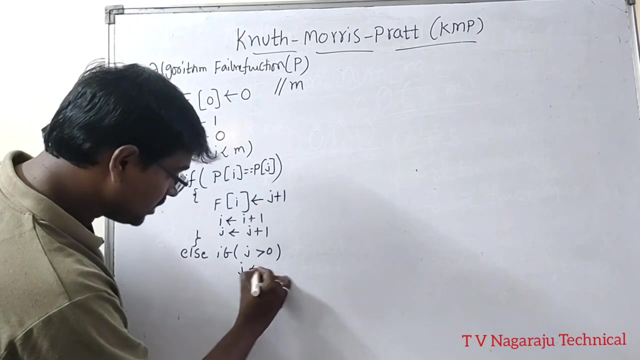 Now check one condition: If j value is greater than 0 or not, If j value is greater than 0 or not, If j value is greater than 0 or not, 0 or not. If j is equal to j. sorry, j greater than 0 means update j value as f of j minus 1.. 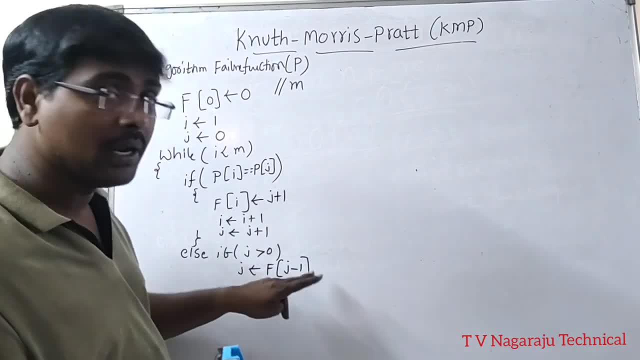 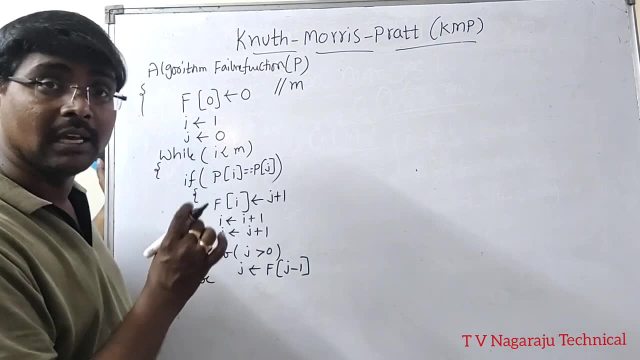 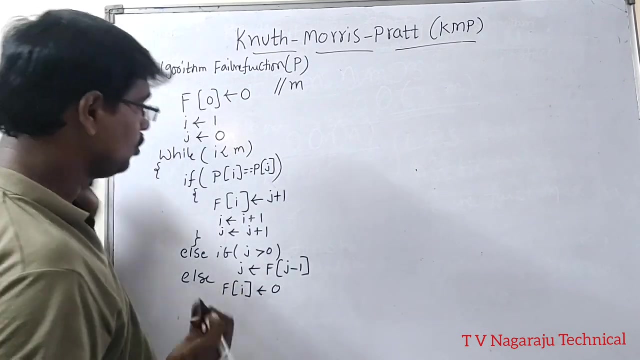 You are not updating any i j is updated to f of j minus 1.. Yes, If this is also fail, if this is also fail, then we are making: f of i is equal to 0.. f of i is equal to 0 and i value. 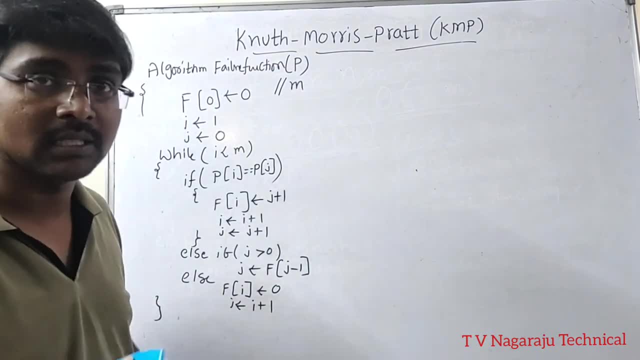 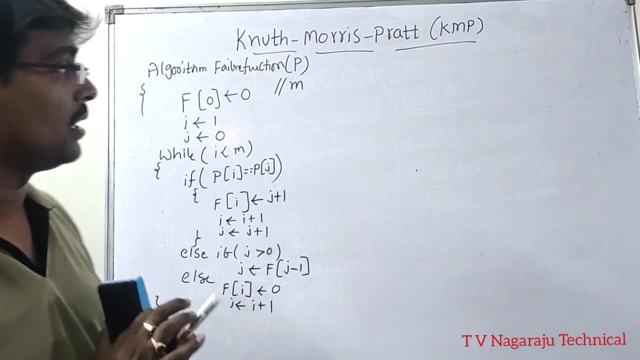 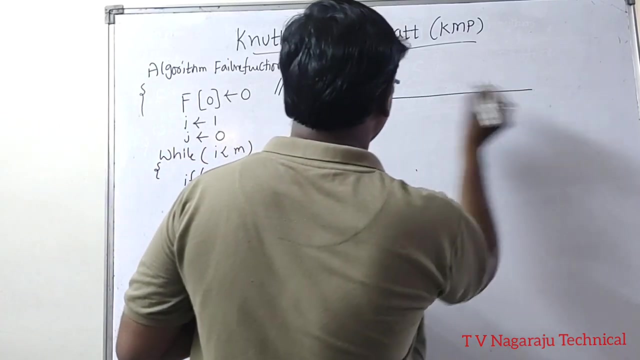 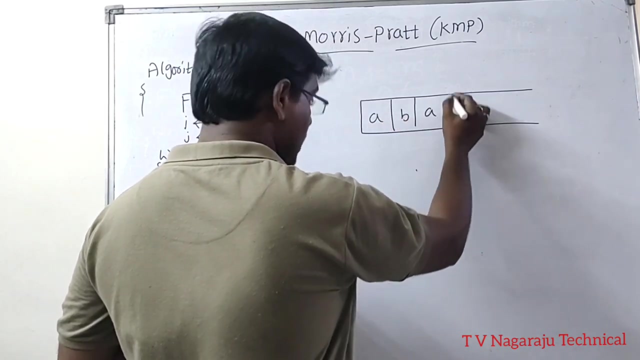 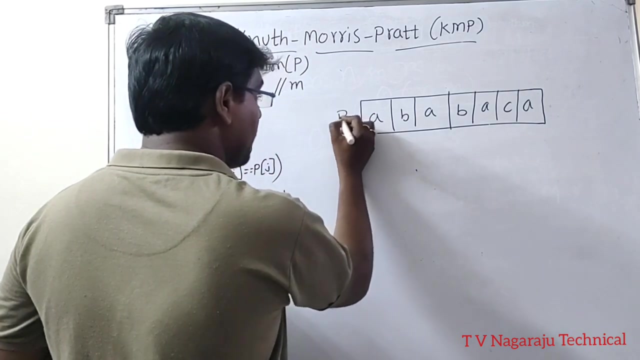 becomes i plus 1.. This is the process. This is the algorithm. Very, very simple algorithm. Once we move with one example, you will get the complete idea. You will get the complete idea. Suppose: consider a pattern. Assume this is my pattern: A, B, A, B, A, C, A. Assume this is my pattern: Index is 0,, 1,, 2,, 3,, 4,, 5,, 6.. 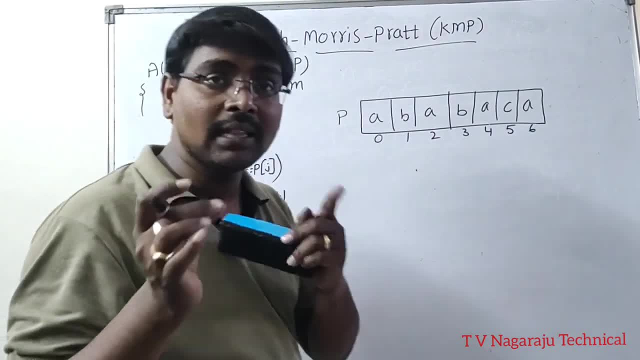 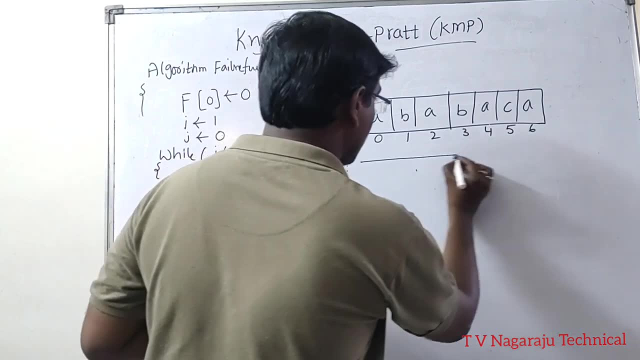 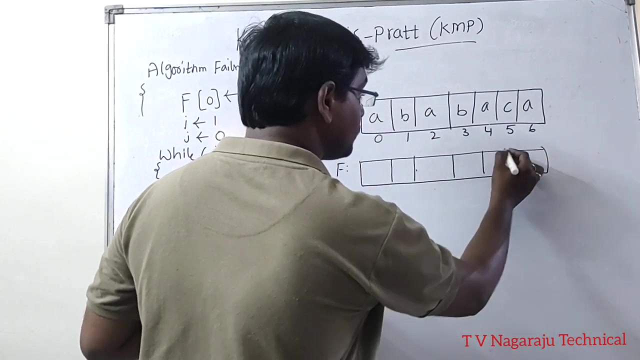 For this pattern, you need to construct the LPS table, also called as failure function. You can use any name, Not a problem. Now, if the size of LPS is also same: 0,, 1,, 2,, 3,, 4,, 5,, 6.. Coming to the algorithm, 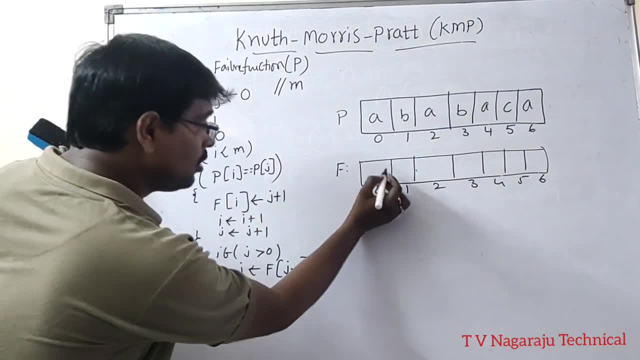 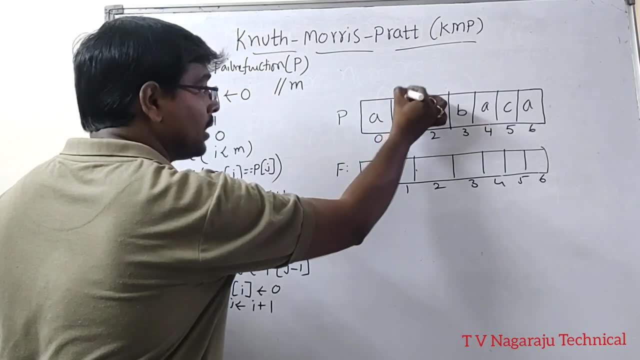 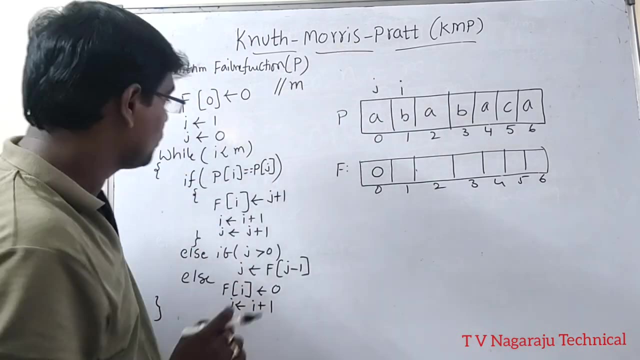 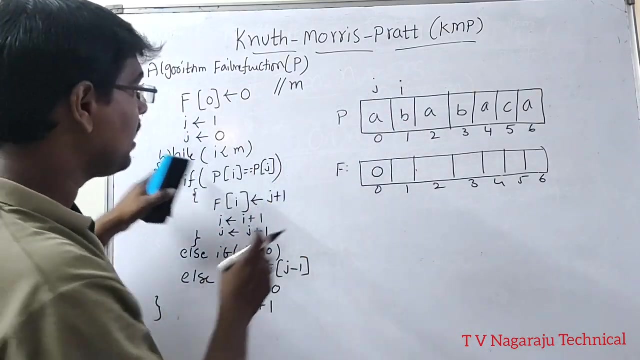 So first, f of 0. At 0th position, fill the value of 0 and initially i is equal to 1.. Suppose i points to this position, J points to this position. Enter into the loop. While i less than m. Suppose 1 less than m value means 1,, 2,, 3,, 4,, 5,, 6,, 7.. 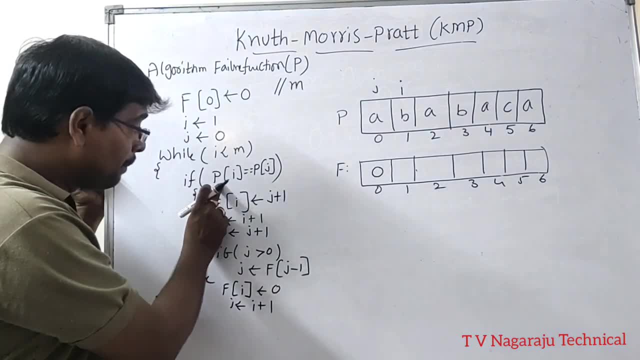 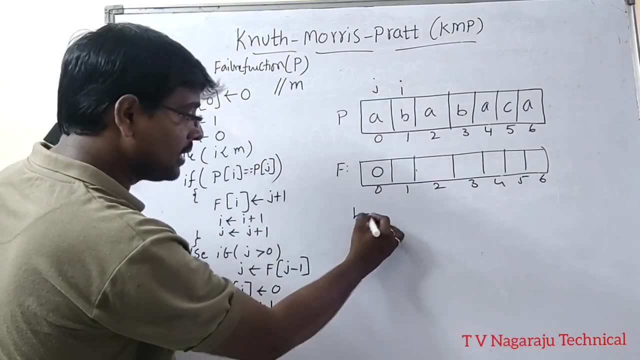 So the length of a string is 7.. Now p of i is equal to p of j, B is equal to equal to a. That is my logic. Now b is equal to equal to a condition. first, If the condition is equal to, if the condition is equal to a, then it is 1.. 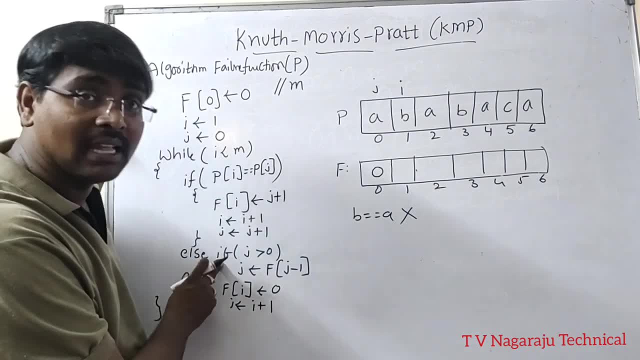 If the condition is equal to, then it is 1.. Now i is equal to, equal to. if the condition is equal to個 with constant full Agr as c 7.. So let us write a Dob prefix false. We are moving into else, if, In the else. if, what is the condition? j greater than 0.. 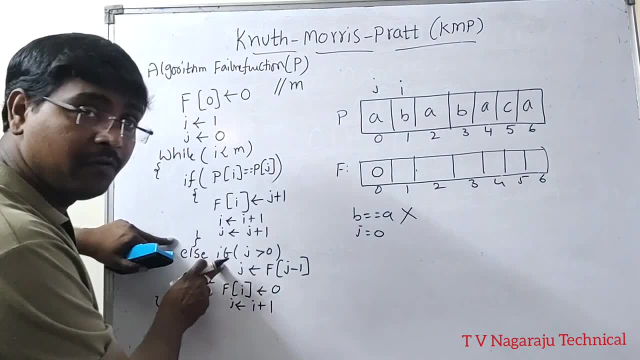 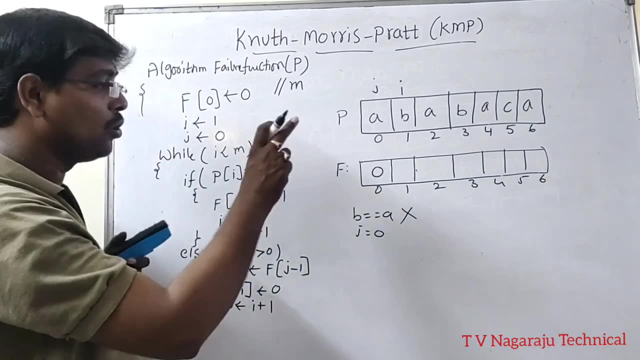 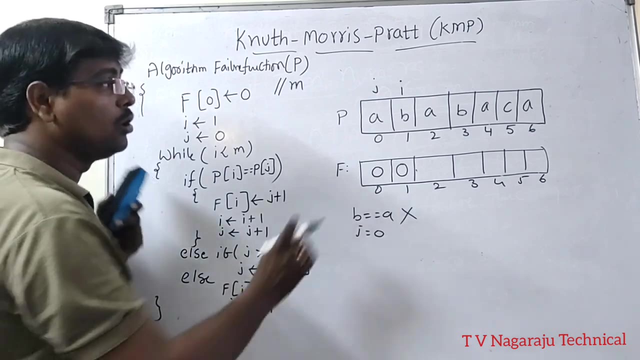 Right or wrong? No, j value 0. Else if is also false, Else In the else we are writing, f of i is equal to 0.. What is the value of i? 1.. f of 1 is equal to 0 and i is equal to i plus 1.. 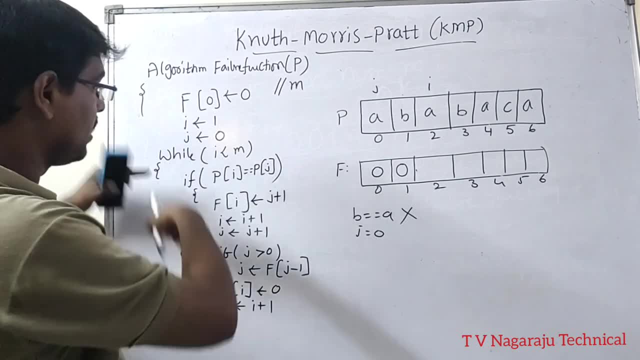 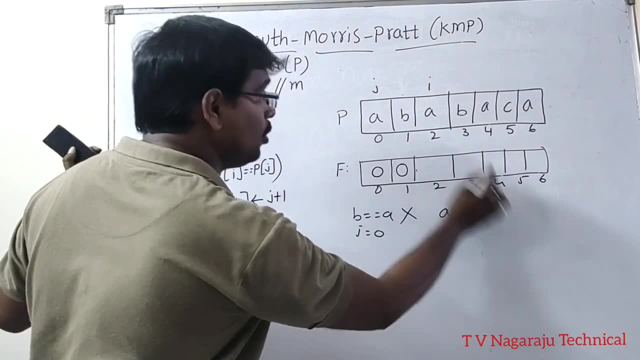 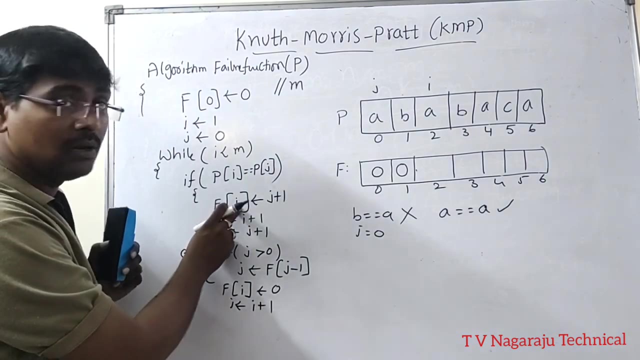 i is incremented Again. repeat the loop. p of i is equal to p of j. a is equal to equal to a Condition true Whenever the condition true: f of i. what is i value right now? 2.. f of 2 is equal. 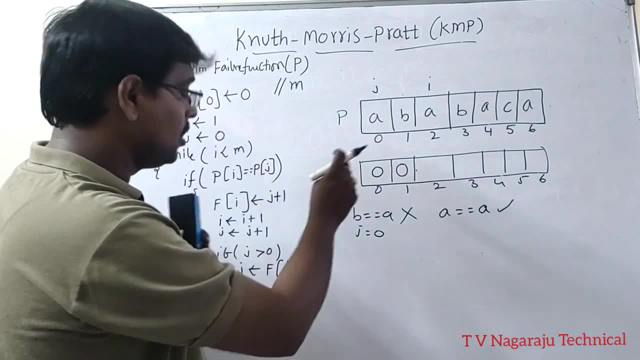 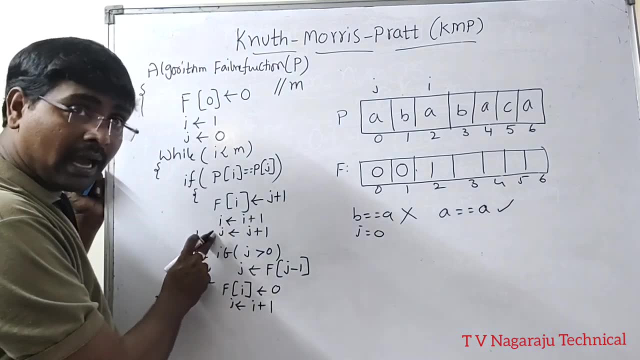 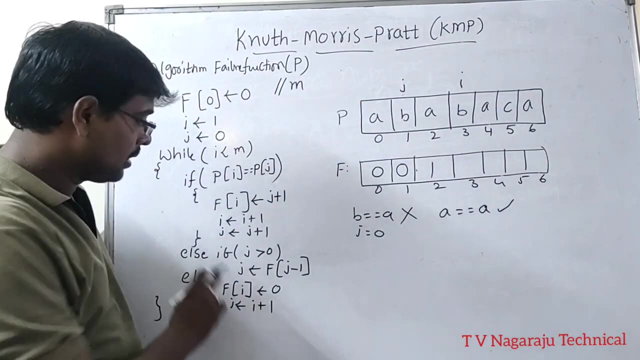 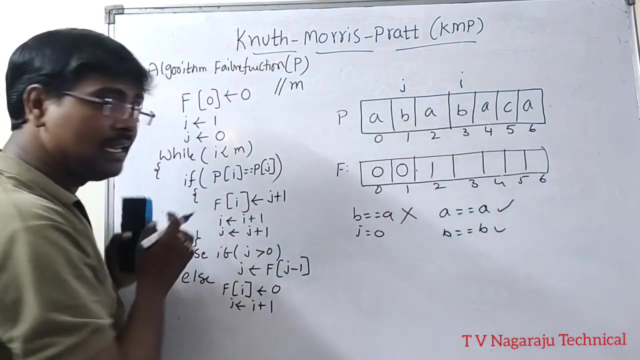 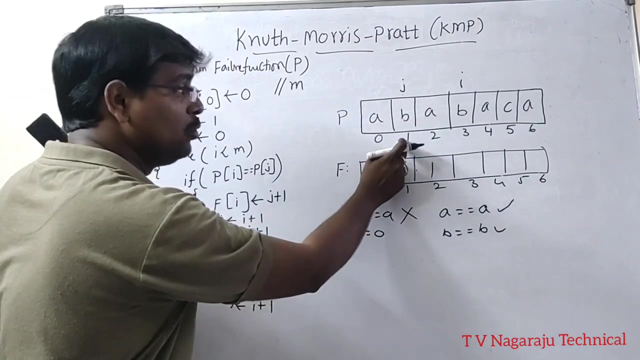 to j plus 1.. j value is 0.. 0 plus 1.. At second position, insert a value: 1.. Increment the i value and j value. j is incremented. i is also incremented. Now repeat: b is equal to equal to b. Yes, Again, the condition is true. f of 3 is equal to j plus 1.. j value is 1.. 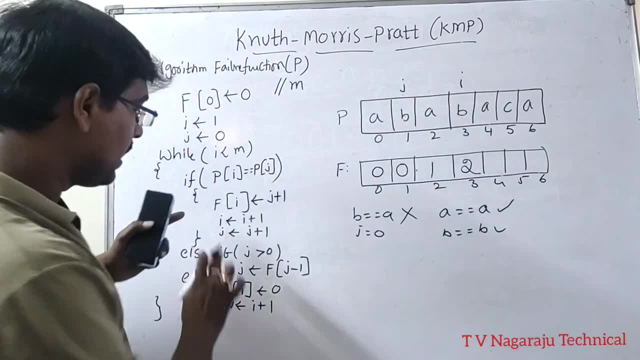 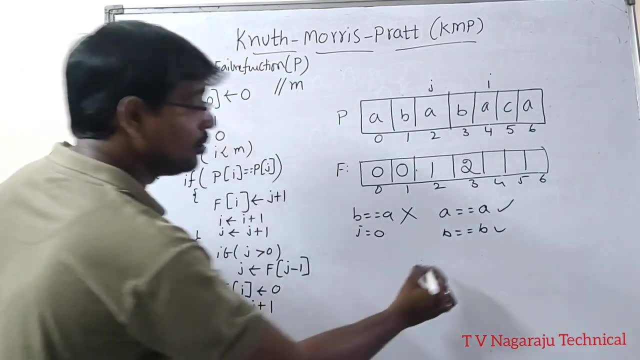 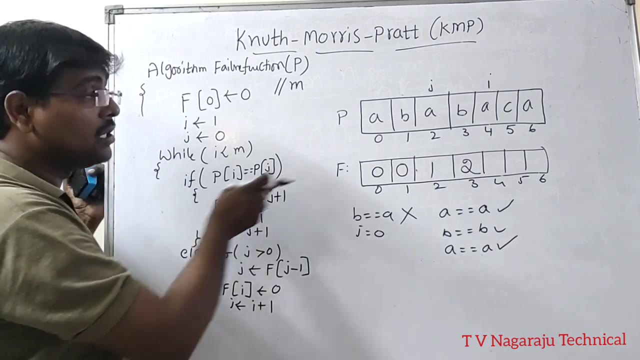 j plus 1 value is equal to 2.. Again, increment: i value and j value j and then i, So a is equal to equal to a. Again there is a match. So f of 4 is equal to. 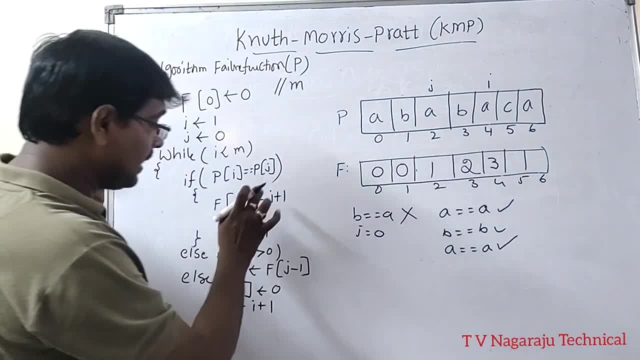 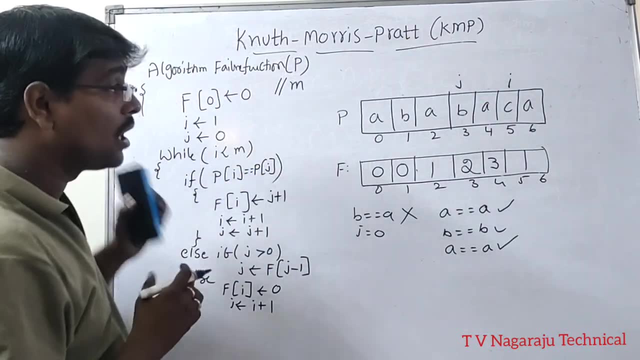 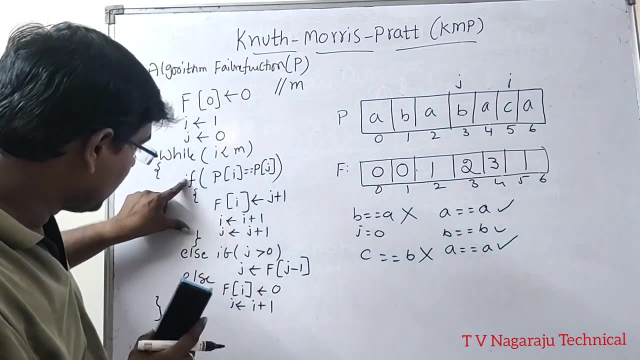 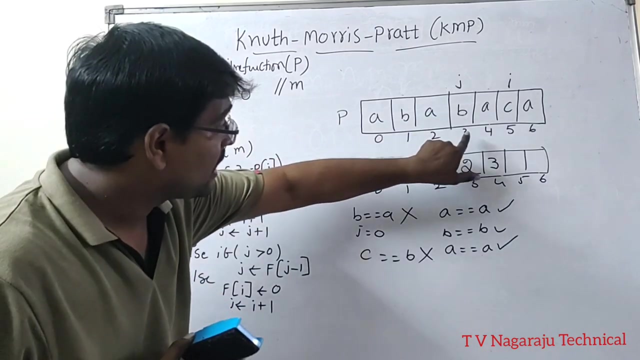 j plus 1,, 2 plus 1, 3.. Increment i value and then j value. i value and then j value. Now c is equal to equal to b. Condition: false: Whenever the condition false, move to. else, if check j is greater than 0 or not, Yes, The j value is 3.. Now what is your step? 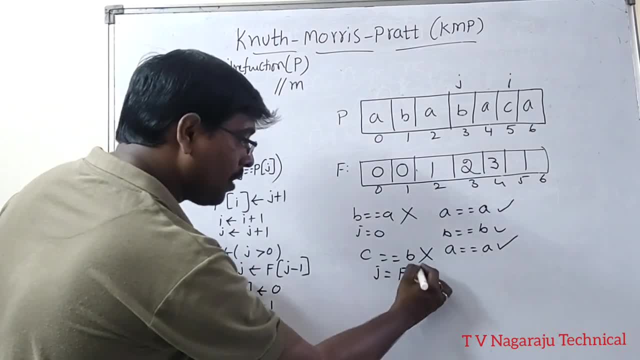 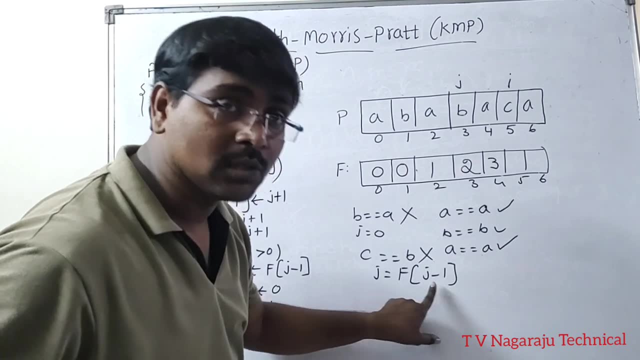 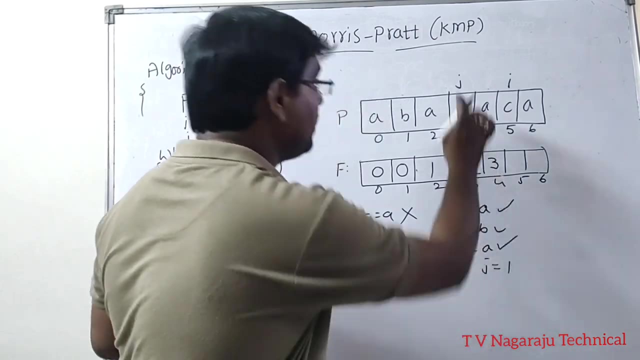 j is updated to f of j minus 1.. j value is equal to 3.. f of 3 minus 1. That is f of 2.. What is f of 2 value 1? Now j is updated with the value 1. j now. 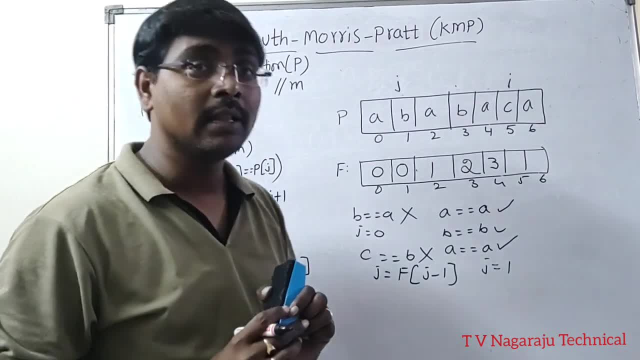 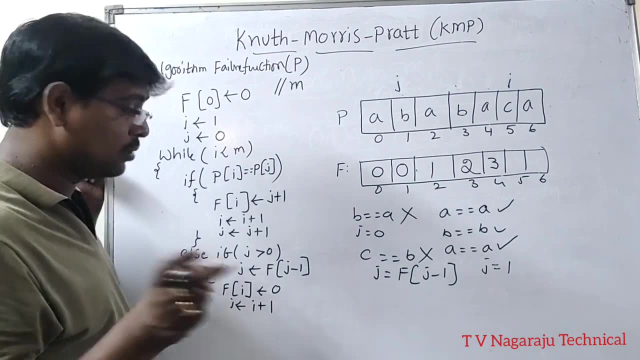 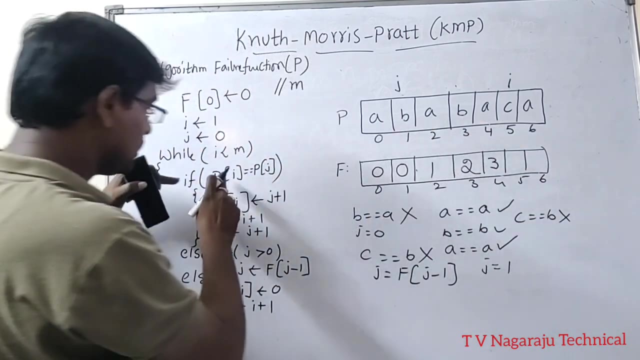 j point to this position. Now. after that again do the comparison Here. I am not updating any. i value Yes or no. Update only. j Now say c is equal to equal to b. C is equal to equal to b- Mismatch. 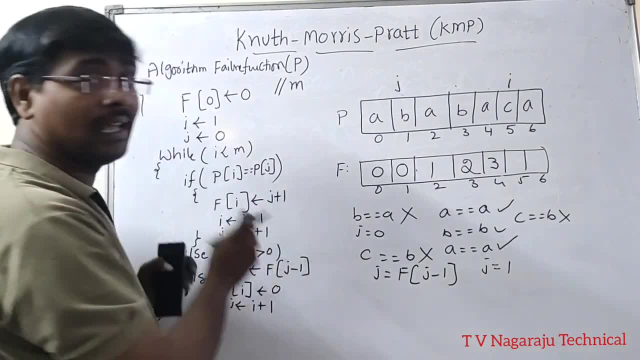 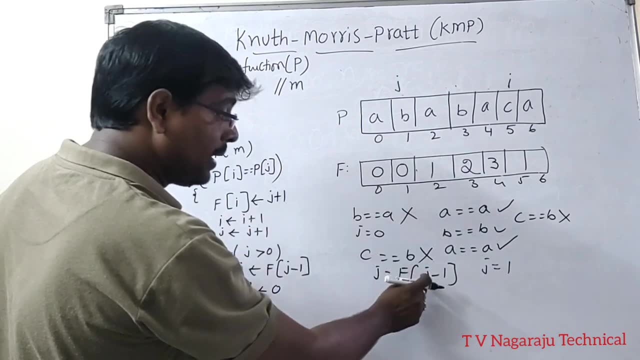 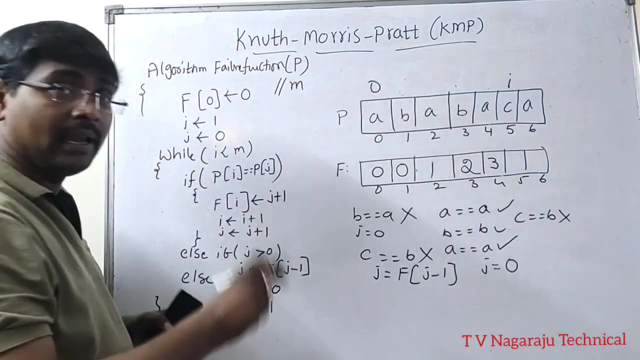 occurred. Move here j is greater than 0.. Yes, Now again, j is equal to f of j minus 1.. Now j is equal to f of j minus 1.. 1 minus 1, 0.. F of 0.. Now J value becomes 0.. Now again, do the comparison C equal to equal to A. 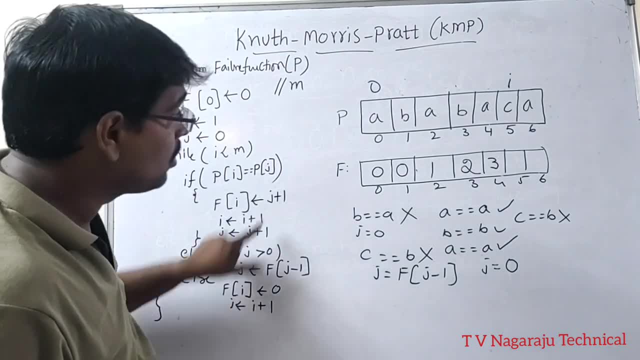 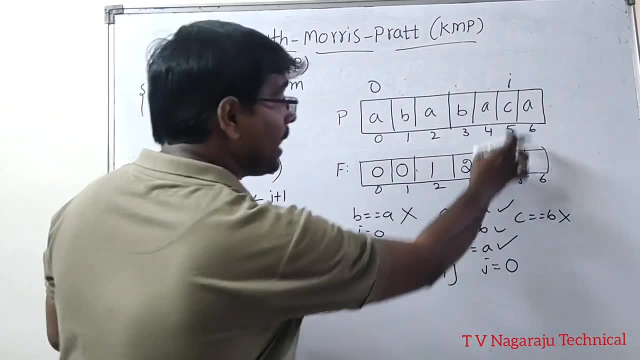 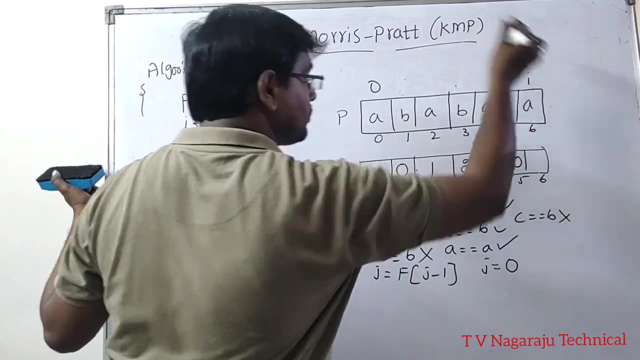 Again the condition fail. J greater than 0,- no, That is also fail. Finally, F of I value is equal to 0.. I is equal to 5.. F of I value: 0.. I is incremented by 1.. Now, in the next step, A is: 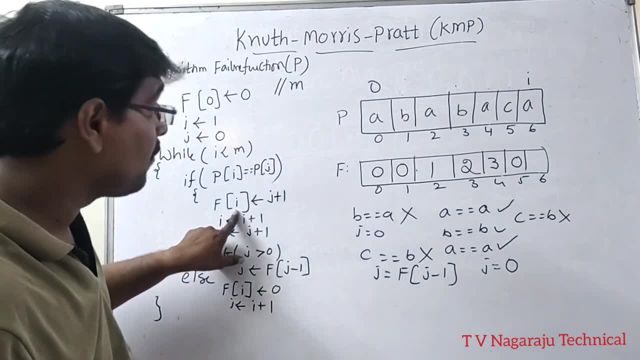 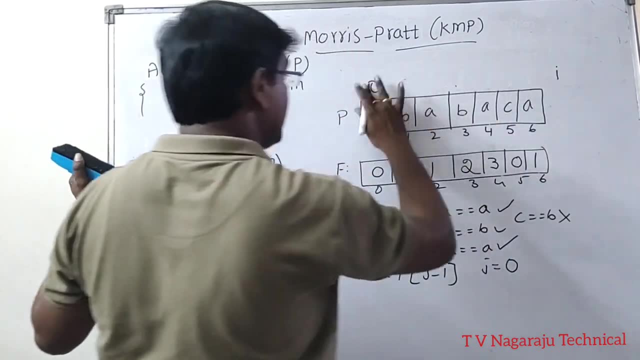 equal to equal to A. Yes, Matching F of 6 is equal to J plus 1.. That is 1.. I is incremented by 1 and J is incremented by 1.. Yes, In the next iteration this condition fail, So I value. 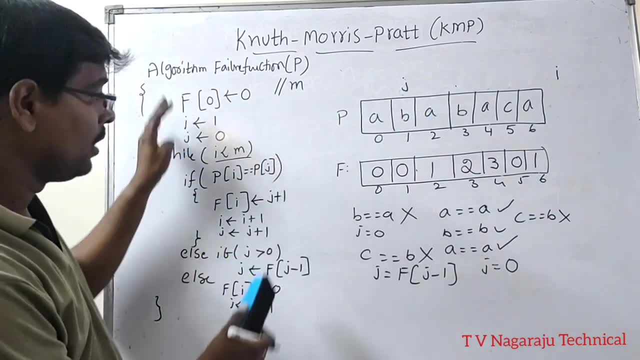 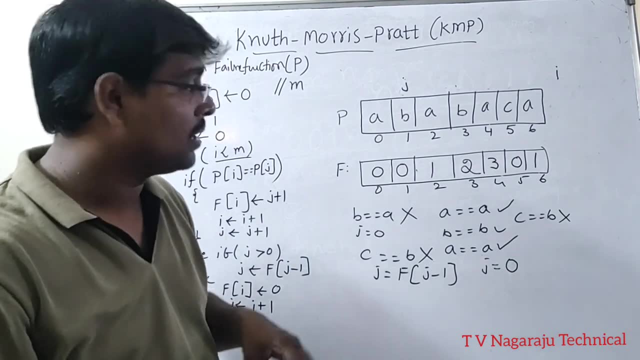 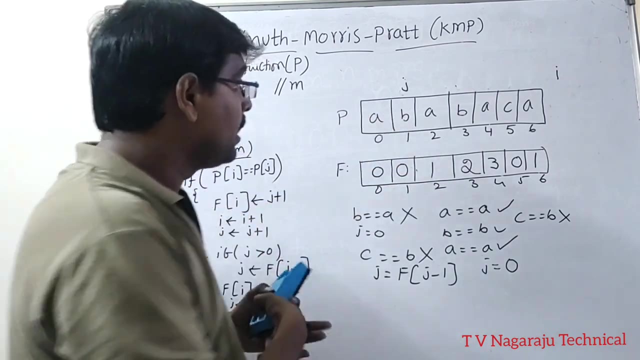 becomes 0. 7.. 7 less than 7 condition fail, We comes out. the LPS table is constructed. Even though you are not knowing the algorithm, it is very, very easy. So very, very easy. First time A appear, 0 times B. Before B appear: No, Now A Already A appear here. 1. B- Continuation. 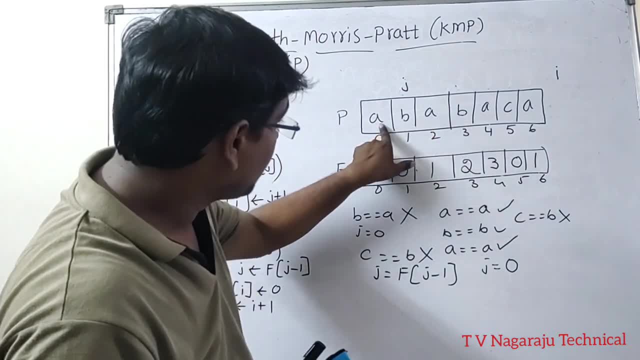 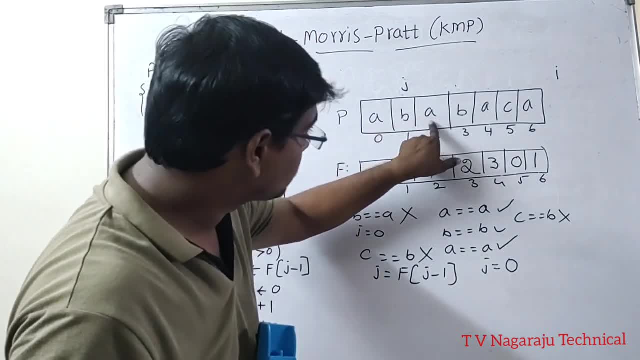 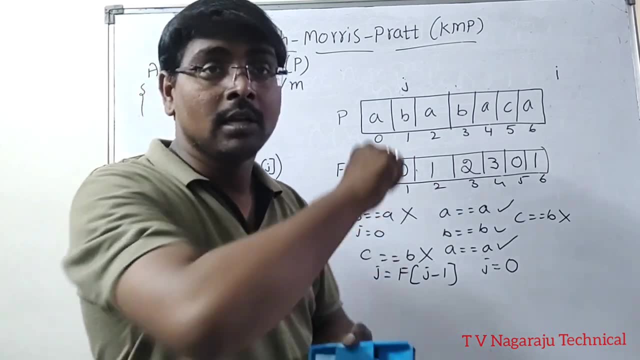 Now B is A, So from the beginning solution: if A is again a, B A, Here also A, B A, so see Not appear before And A again appear. I think you got me. So if the pattern is repeated, 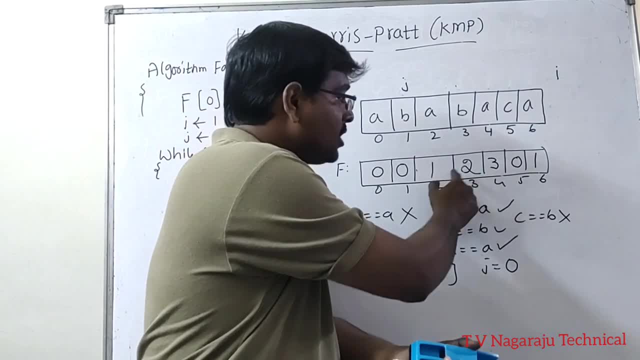 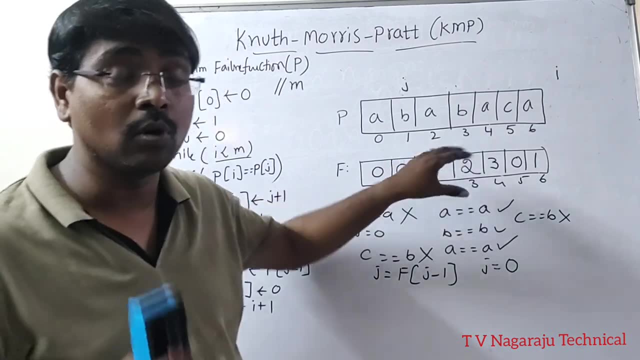 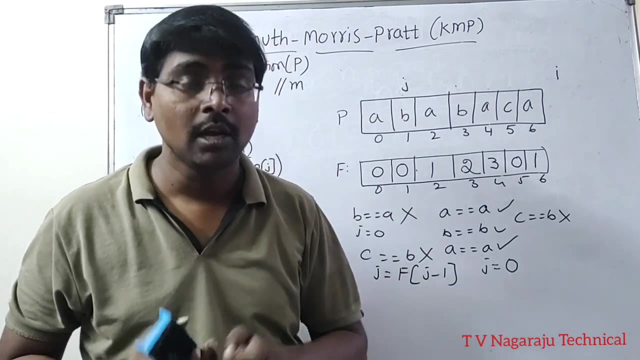 According to the repetition, We are increasing the value. So by using this function, we are constructing the LPS table. We have another way, also By using the concept of proper prefix and proper suffix. You can do it, you can make it. You have to create 예�ing. if not, you can. 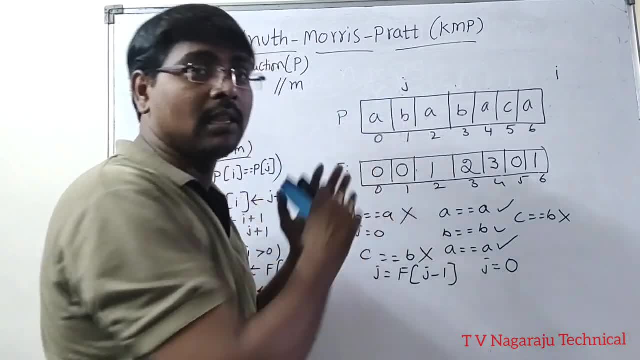 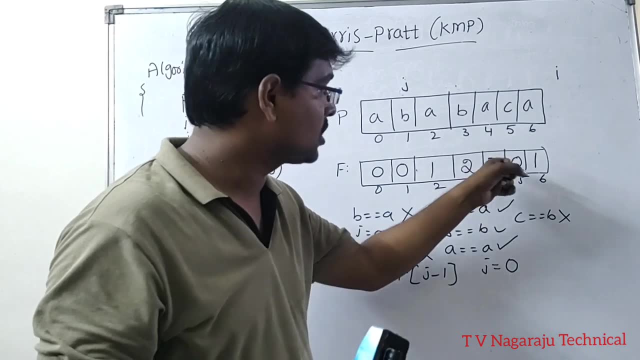 ci, e swaying, using proper prefix and suffix, or you can do this: Hm, hmm, Or as another, anyway. anyway, in the next video we will move to that way, that is, lps table construction without using this function, a simplified way of constructing lps table. we will discuss that thing. 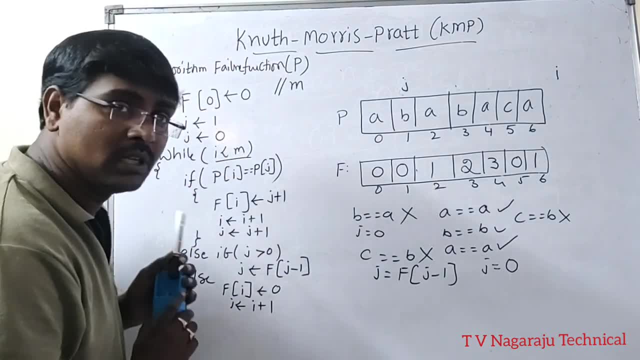 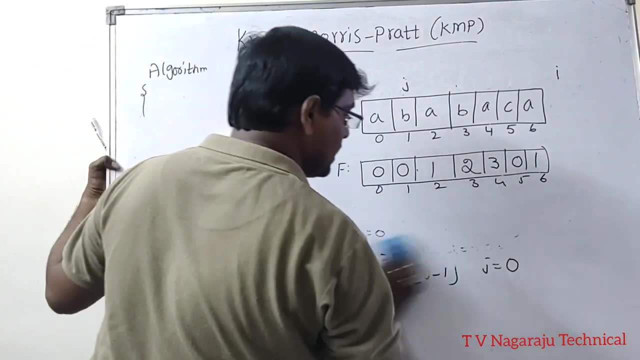 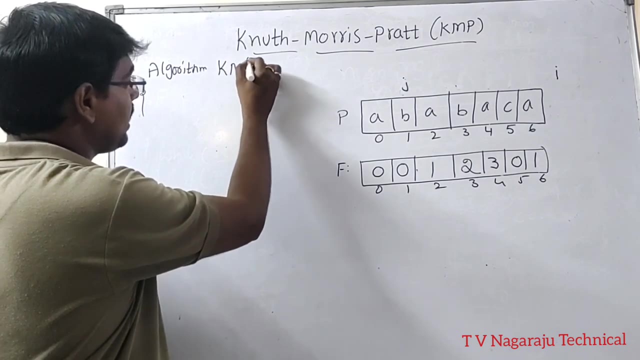 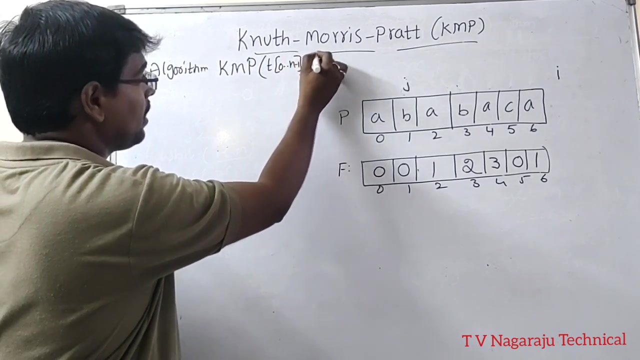 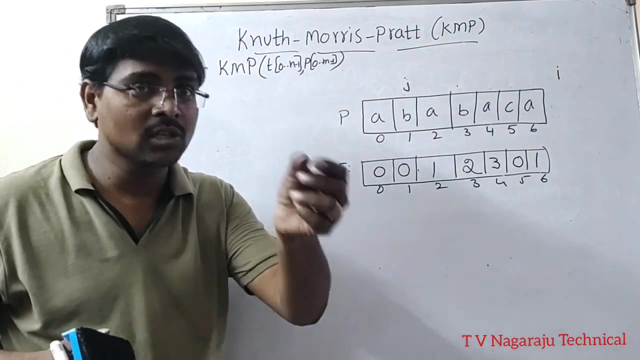 also in the next section. now lps table is constructed successfully. what is the next step? obviously, the next step is kmp algorithm. kmp algorithm. write down the kmp algorithm of suppose text 0 to n minus 1 comma, pattern 0 to m minus 1. so two parameters, one is the text. 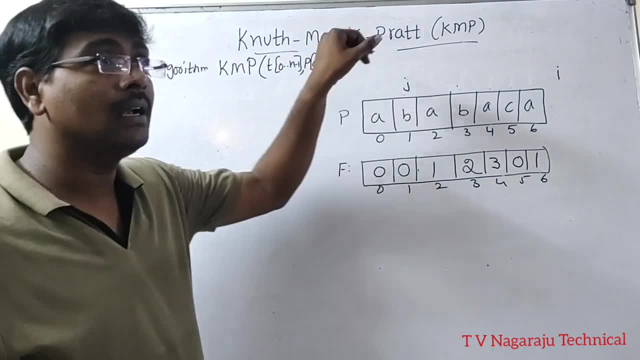 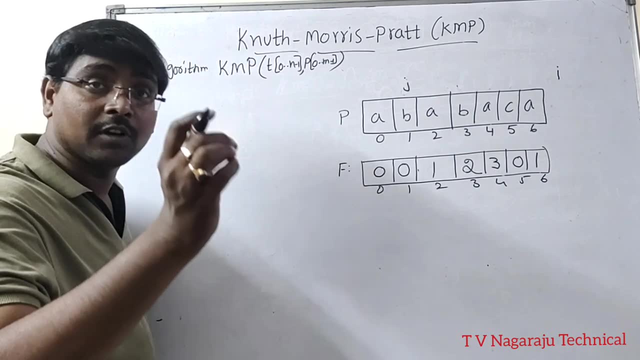 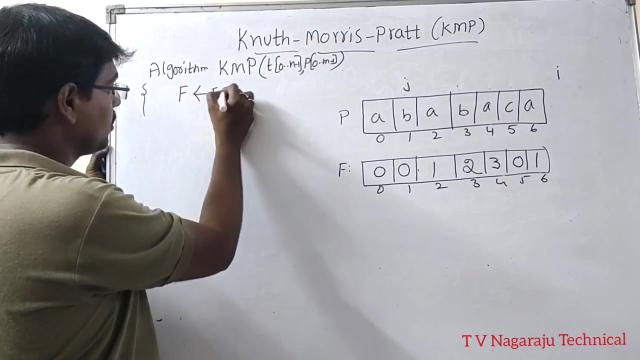 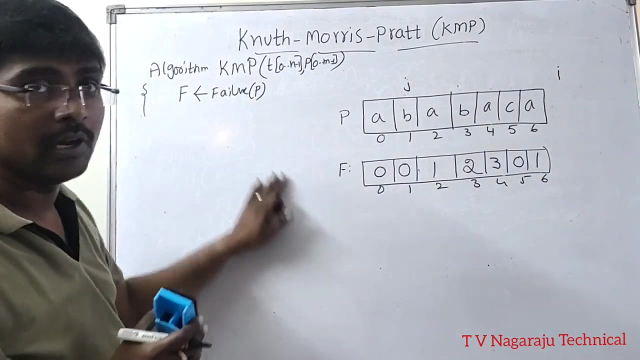 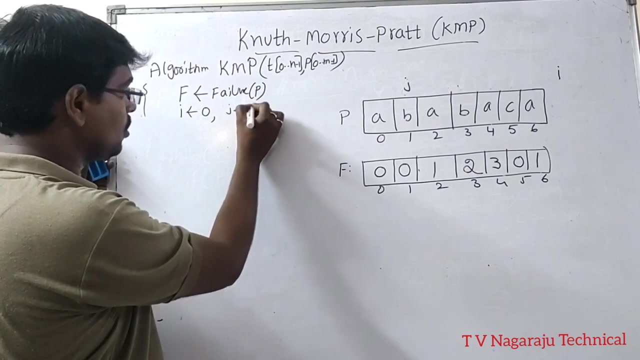 of length n. another one is the pattern of length m. okay, what is the first step of the kmp? already you know the first step is calculation of failure function. so f tends to failure of p. so for the pattern, i calculated the failure function. now i am taking two parameters: i equal to j, j is equal to 0, i equal to 0, j. 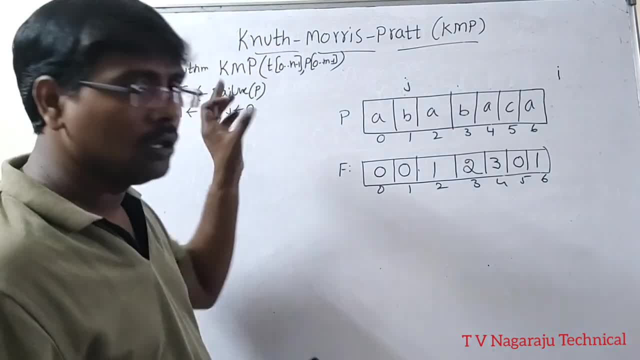 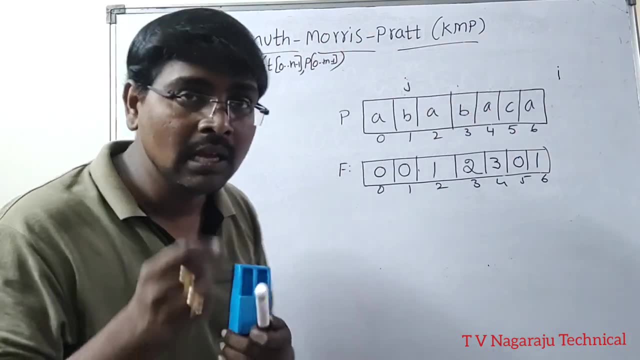 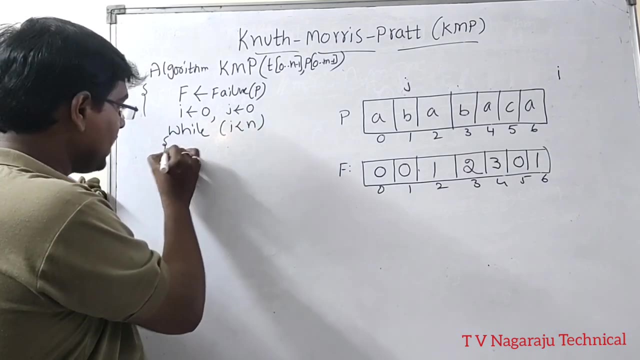 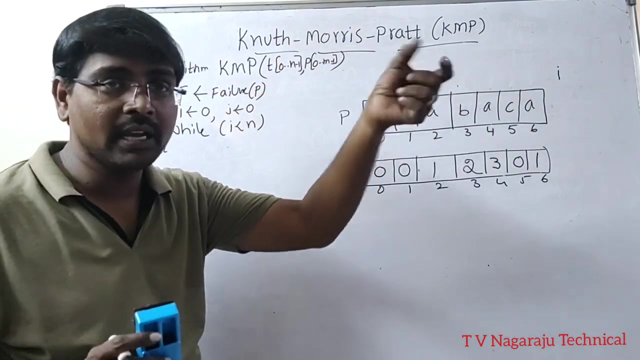 is equal to 0. simply, i is used to traverse the text, j is used to traverse the pattern. to traverse the pattern now, while i less than n until the end of the pattern. what is the first step? compare the first character of the text with the first two character of the pattern. if there is a match, move to the next. 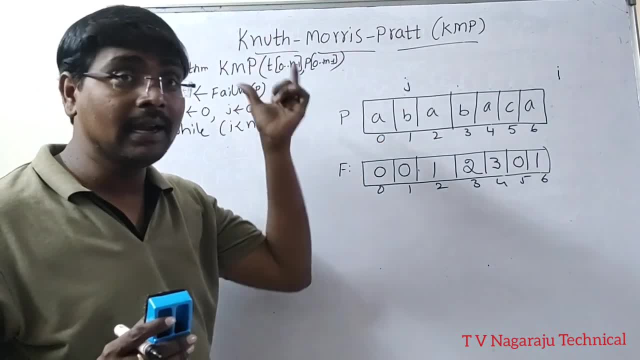 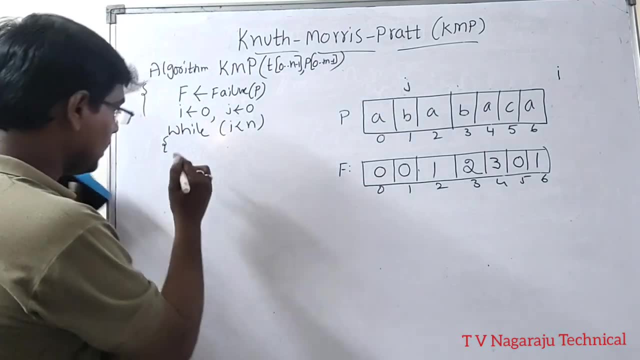 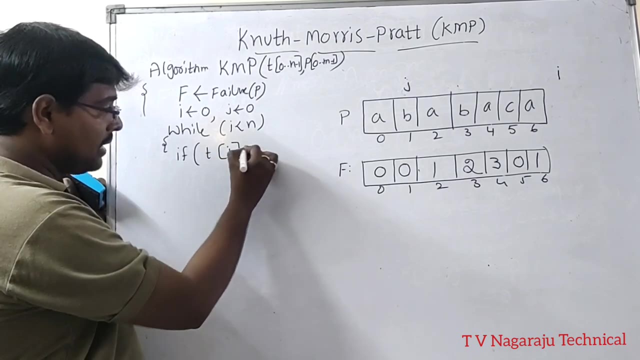 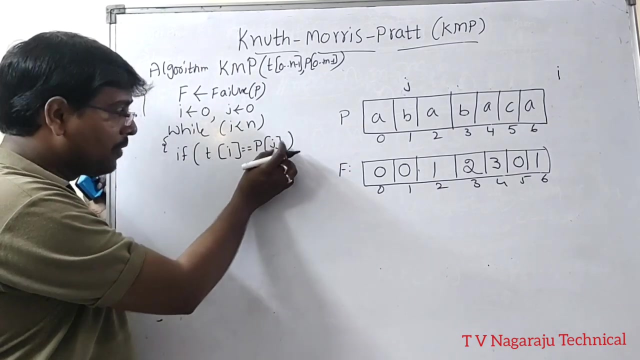 If there is a match, move to the next position. If the entire pattern is completed, the particular pattern is available. return the index. Exactly, that is my first step. What is my first step? If t of i is equal to equal to p of j within the while loop, if t of i is equal to p of j, if both are equal, we are checking one condition. 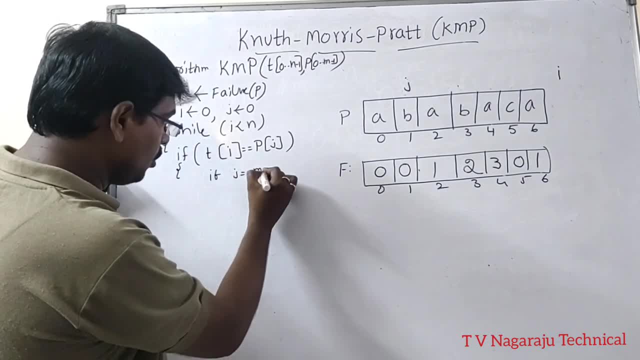 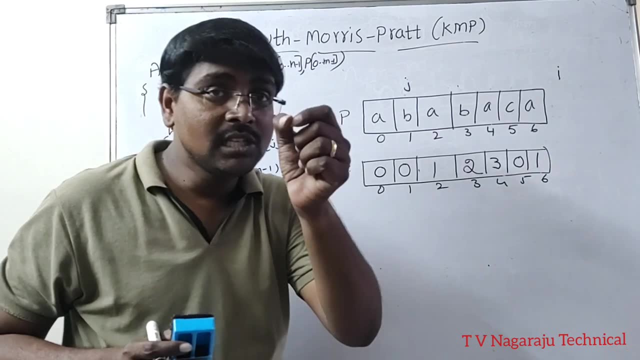 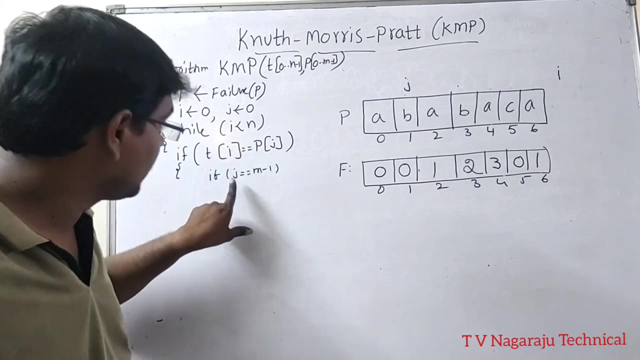 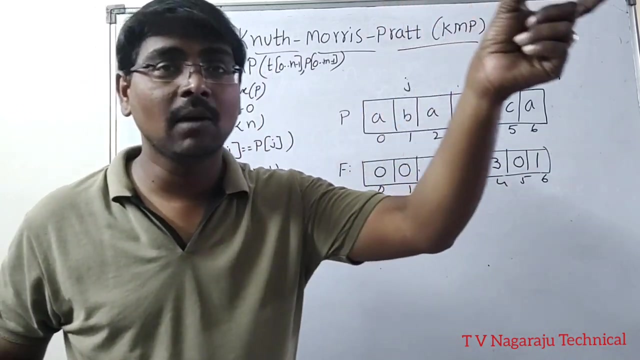 If j is equal to equal to m minus 1, what is the meaning? j equal to m minus 1, I said j is used to traverse the pattern. If both the characters are equal and at the same time j is at the last position means my entire pattern is available in the given test. 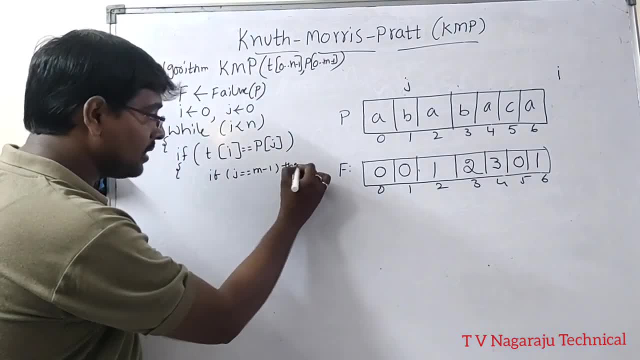 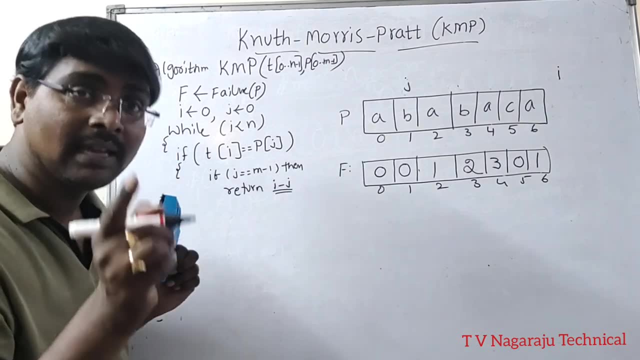 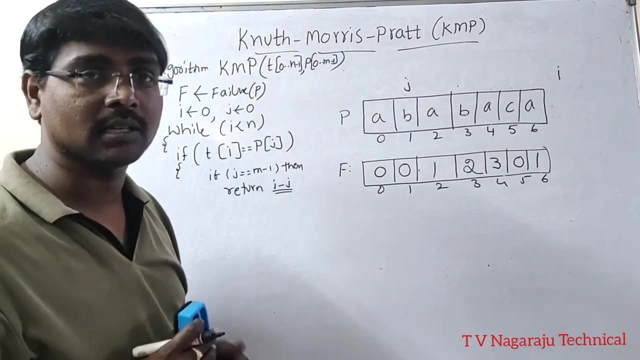 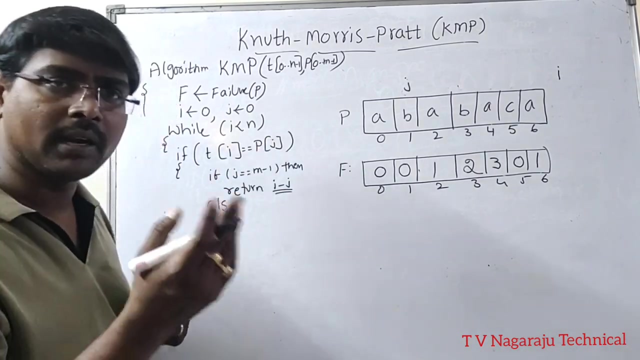 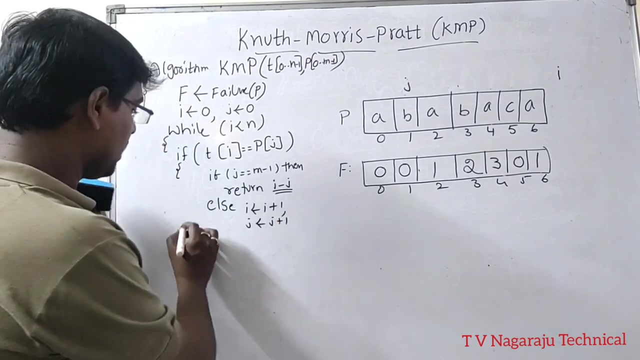 Yes or no. If this is the condition, then you need to return i minus j. What is i minus j? The answer, that is the index. where the pattern is available, then the algorithm is completed Exactly, Successfully, For example, even though there is a match, but the end of the pattern is not reached. What happened? Simple procedure: Increment the value of i by 1, increment the value of j by 1.. 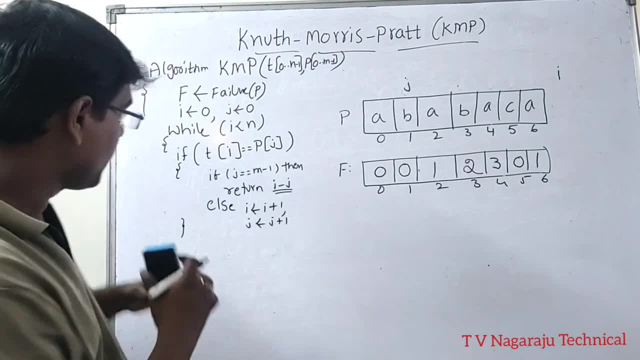 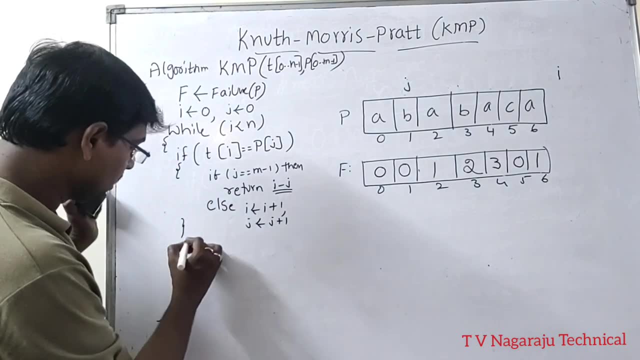 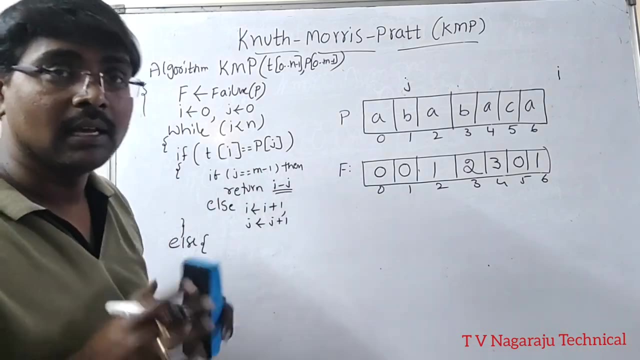 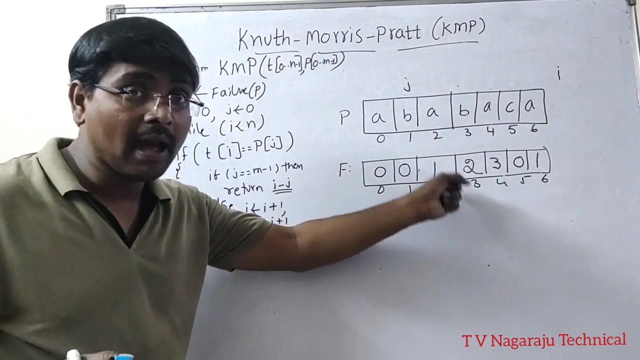 For next element, comparison. For next, character comparison. This is the thing. if the characters are matched, Obviously, what is the another one? Else, Else. in the sense, if the characters are matched, then the algorithm is completed. If the characters are not matched, then what you need to do, You need to go through the LPS table. According to the values of LPS table, you need to skip the comparison of the characters. 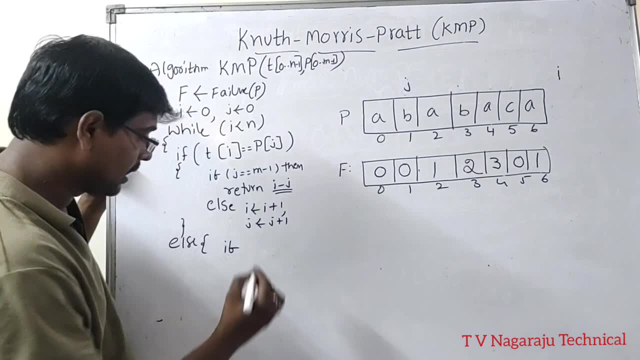 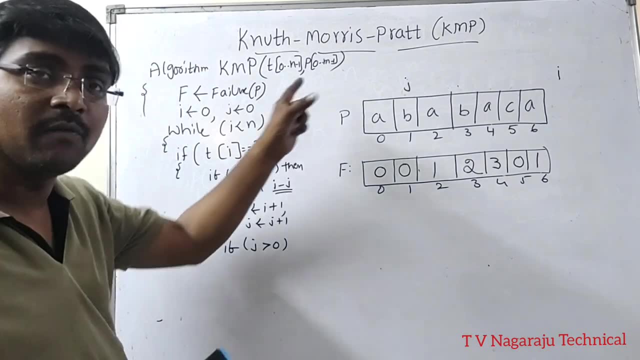 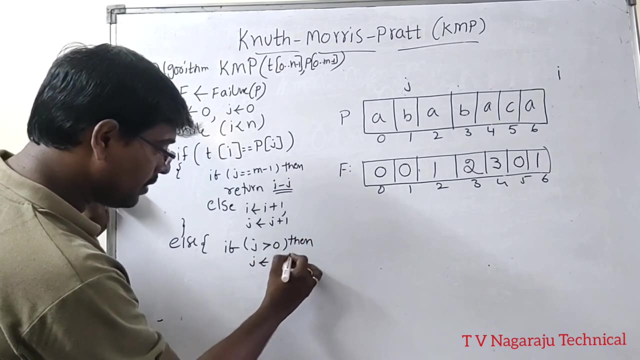 So yes, here we are checking one condition: If j value is greater than 0,, whatever the logic we written in failure, here also same logic: j greater than 0. So j is updated with a value of f of j minus 1.. 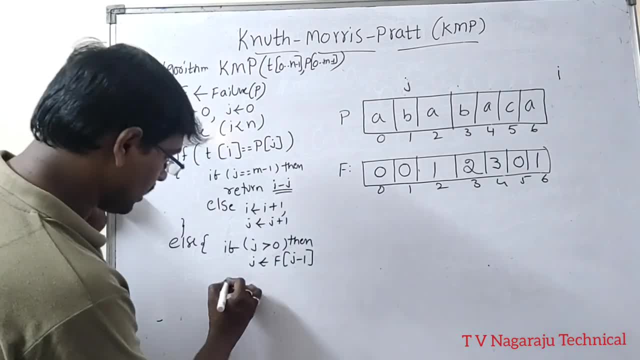 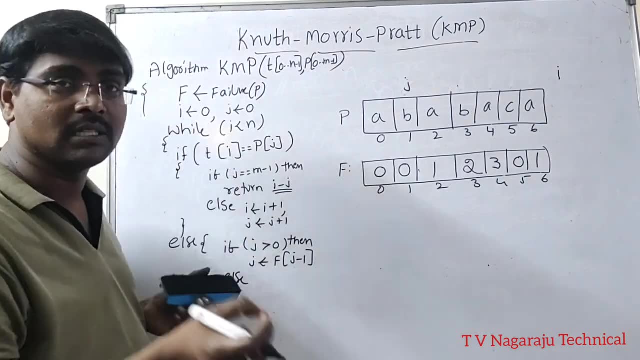 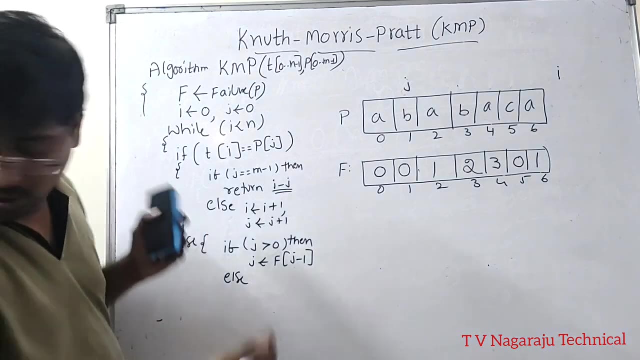 j is updated with f of j minus 1.. Suppose else For this. if else Else means j greater than 0. False, That means j value is equal to 0.. If j value is equal to 0, simply i is equal to i plus 1.. 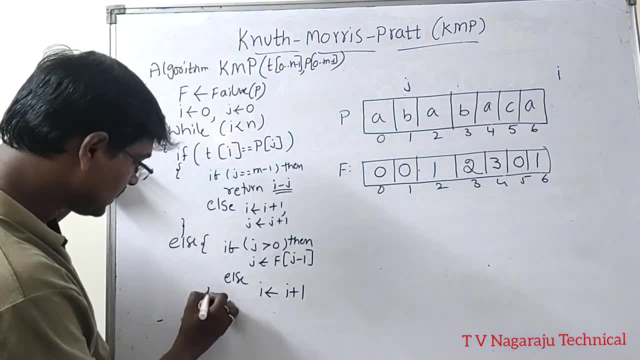 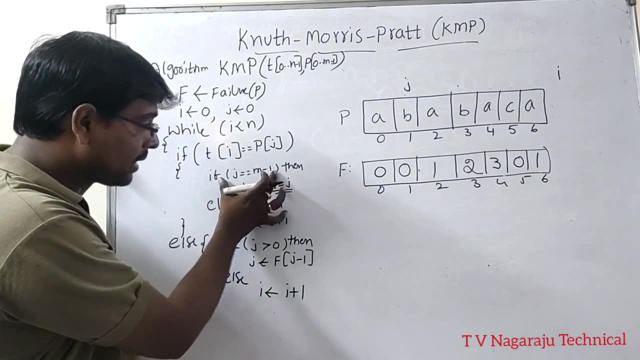 Move to the next character. Okay, This is else case. If case means if there is a match. if there is a match, if the end of the pattern is reached, return the index. If the end is not reached, increment Suppose if there is no match. 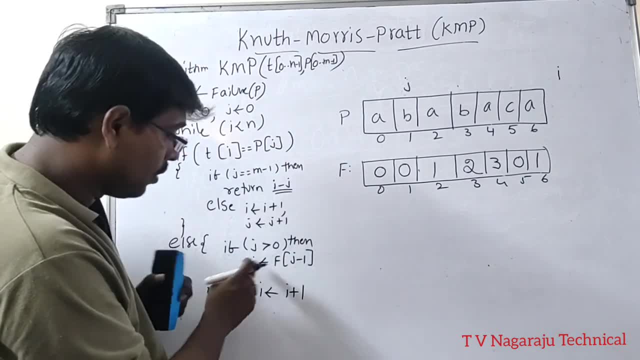 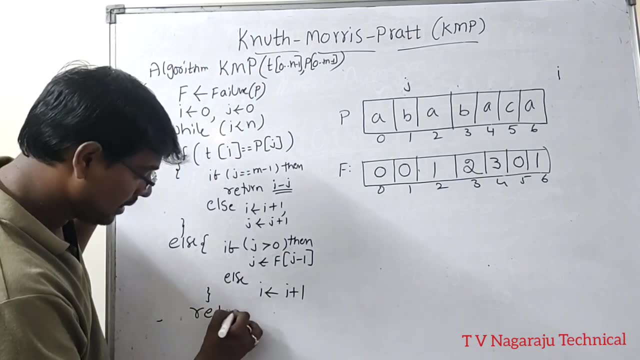 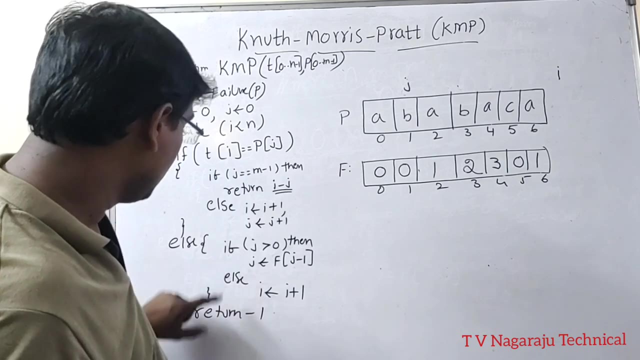 if there is no match, use the LPS table. The pattern is updated. Pattern is updated. Now, finally, return minus 1.. So, in the entire table, in the entire table, if all are failed, return minus 1. return minus 1 in the sense. 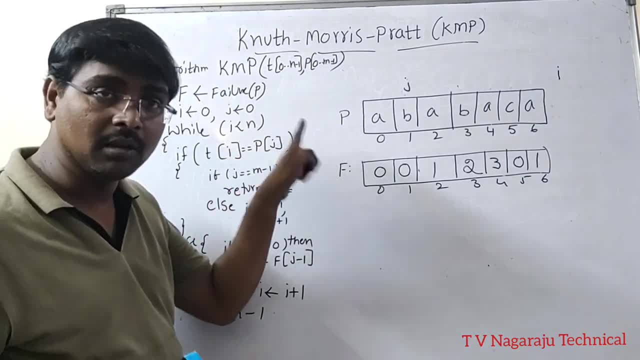 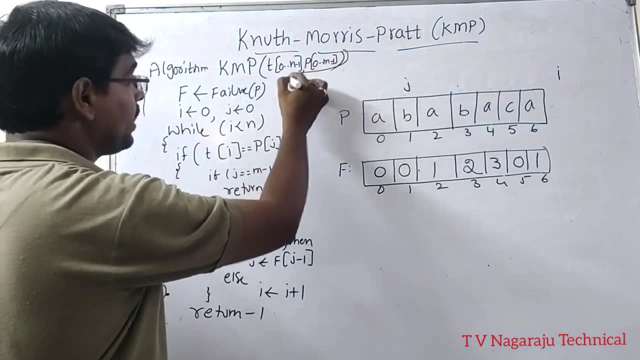 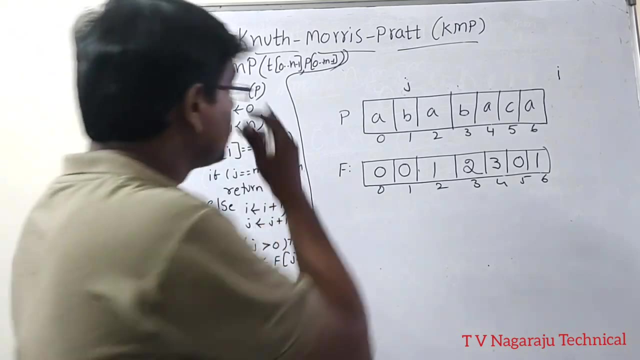 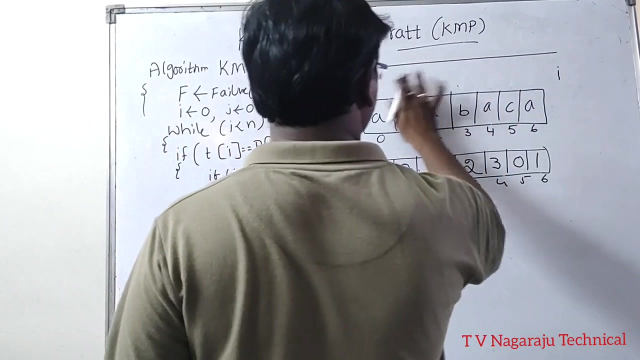 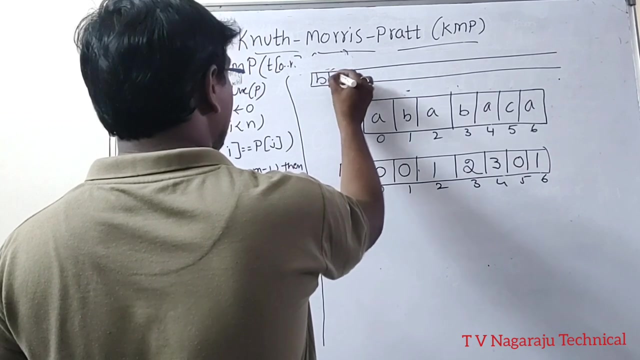 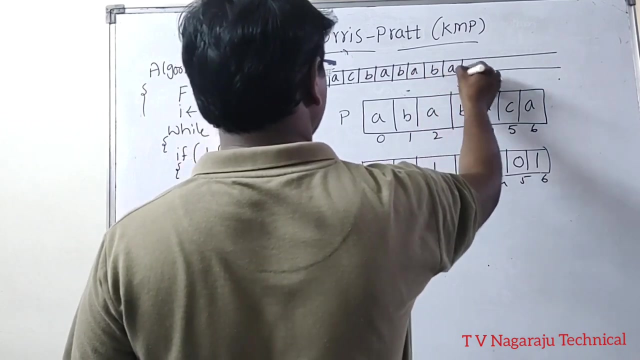 we are coming out of the loop. the entire pattern is checked. there is no match. there is no match. okay, now i will implement one example. implement one example for this kmp algorithm. suppose consider one text b. i will write down in boxes: b a c, b a, b, a, b a, b, b a c. 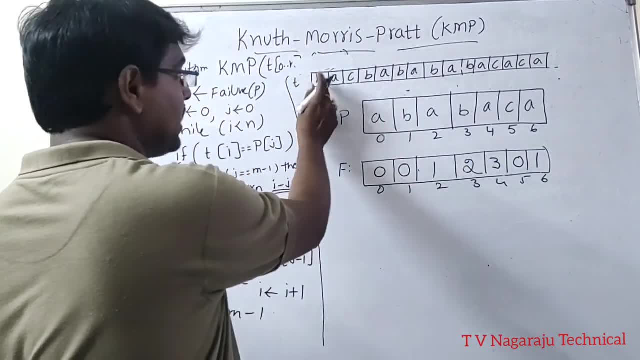 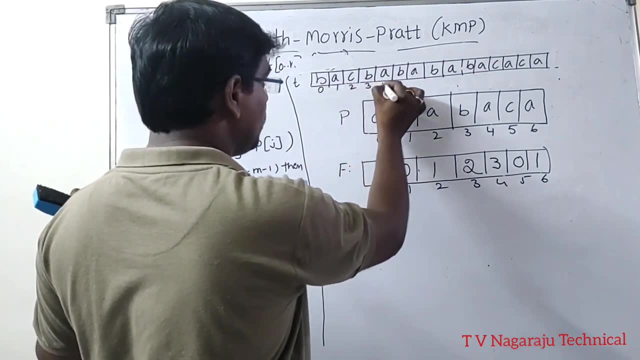 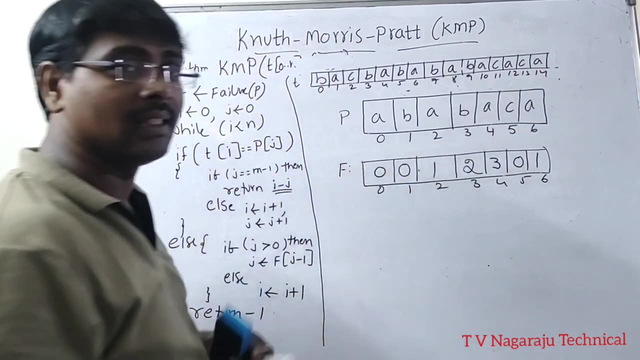 suppose i will take this text. this is the text: pattern and failure function or lps table. write down the indexes also: 0, 1, 2, 3, 4, 5, 6, 7, 8, 9, 10, 11, 12, 13, 14. 15 is the length of the pattern. 15 is sorry, 15 is the length. 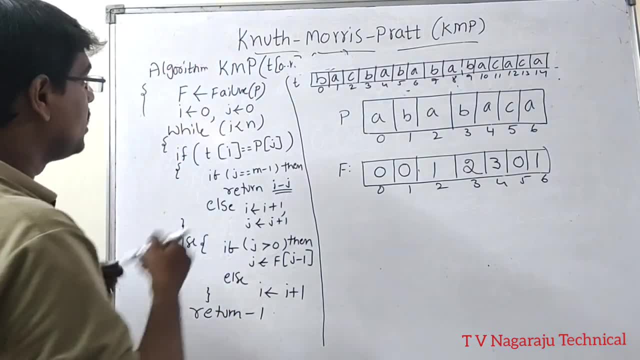 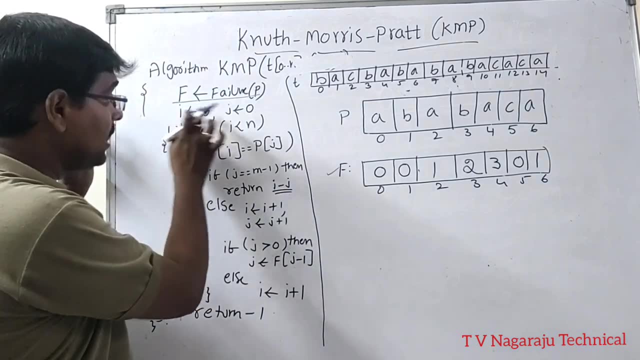 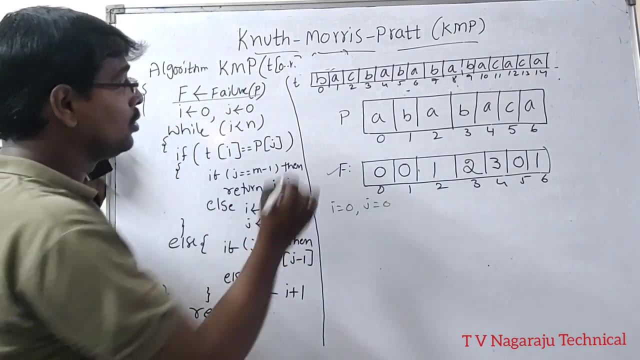 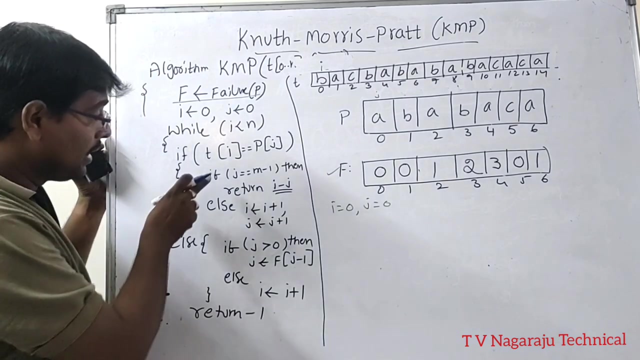 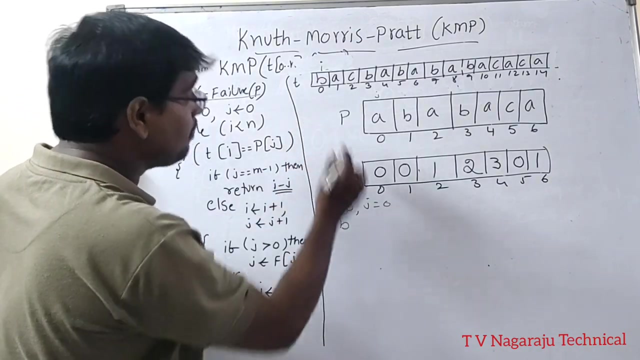 of the text. now follow step by step. so what is the first step? calculation of failure table. yes, completed successfully. när det is equal to equal to a condition false. whenever the condition false, we are moving it in a transactional way. finally, we will go back to the basic methods. this time we are going to work on second layer value under 같은 subir. i will write down here: i is equal to equal to zero. now, this is i value and this is j value, yes or no or no, but here, if or no, here is equal to equal to to p of j. what is ksi is equal to, equal to a condition false. whenever the condition false, we are moving it in a مسwny way, as you see here. we have to move it in a moving pattern here. 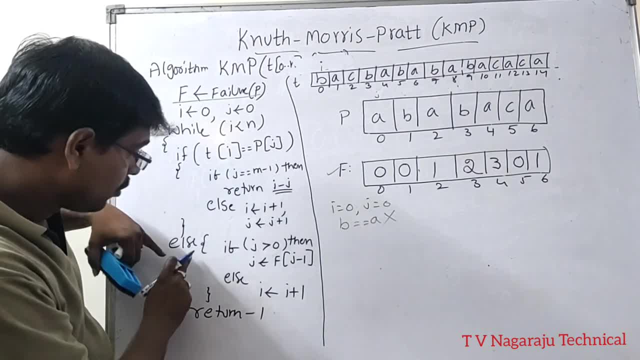 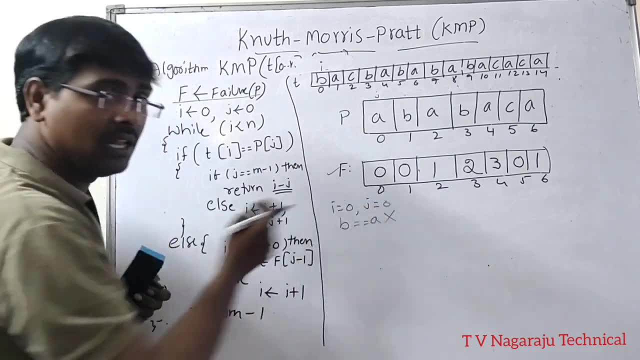 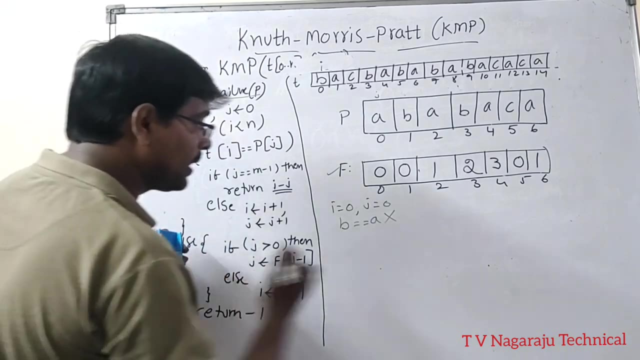 Whenever the condition falls, we are moving into else. We are checking: j greater than 0, Yes or no? No, j value is equal to 0. If also fail, else, i is equal to i plus 1. Now what happen? i value becomes 1. 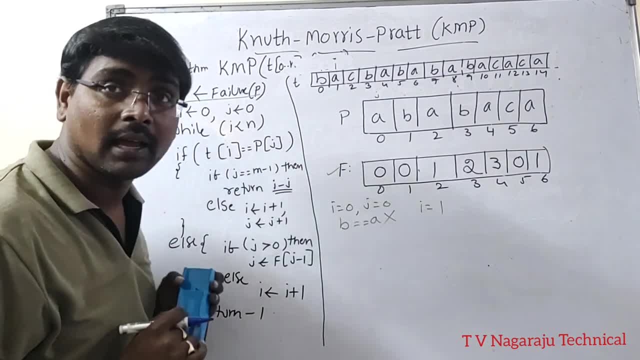 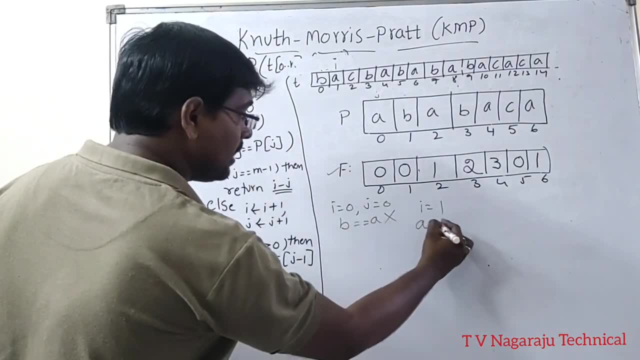 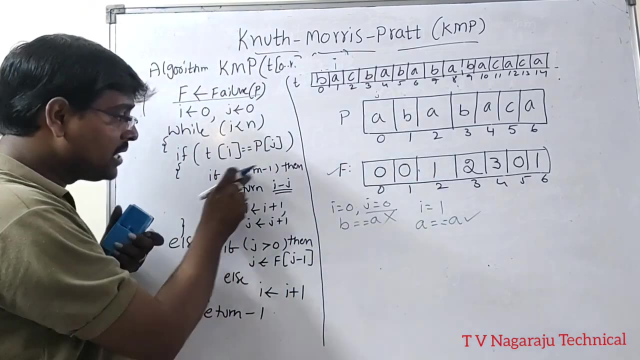 Now i moves to this position. i moves to this position Again: t of i. t of i means a is equal to equal to j, is not updated a, Both are equal. And is j is equal to m minus 1?? No, j value is just 0. 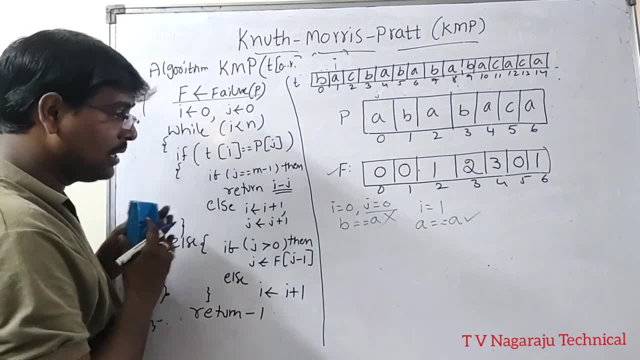 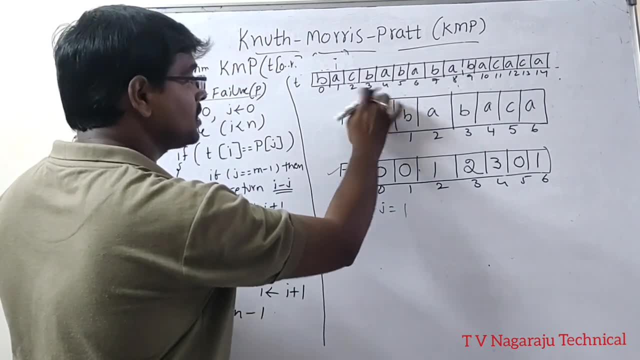 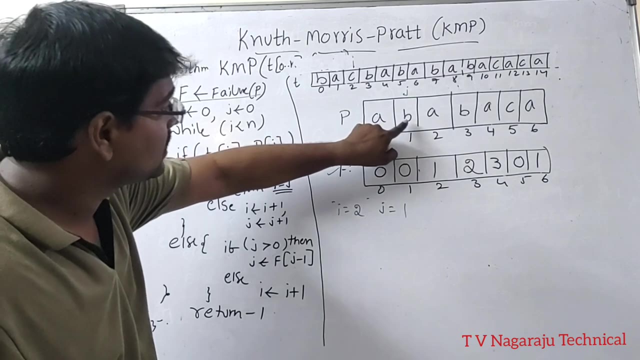 Now i is equal to i plus 1. j is equal to j plus 1. Now i value becomes 2, j value becomes 1. This is j, this is i. Now compare the character. c is equal to equal to be. No, c is equal to equal to be. 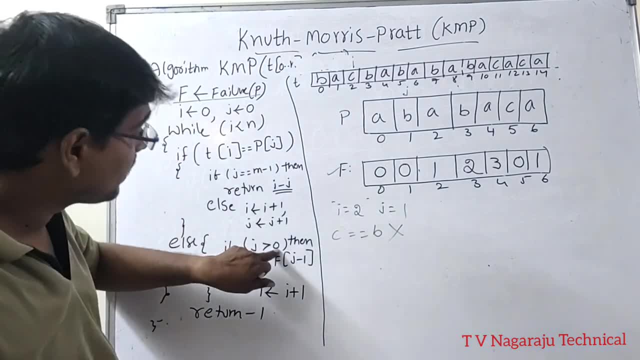 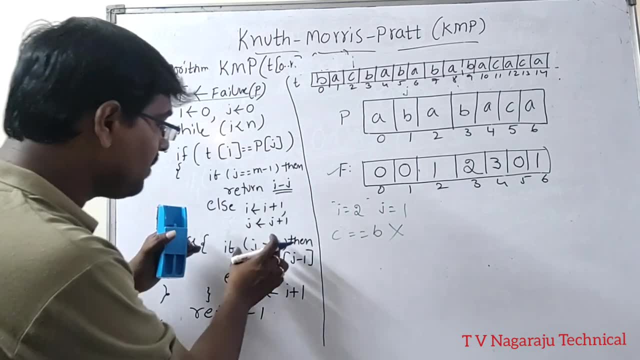 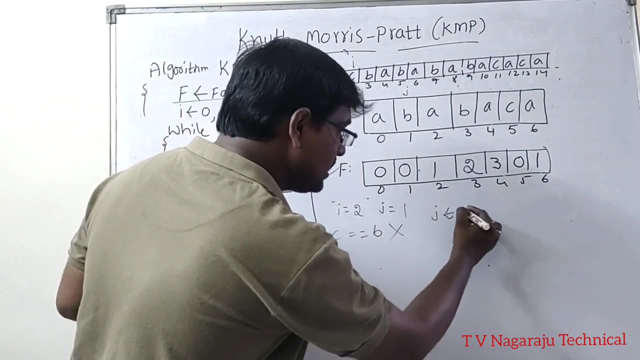 No, Come into else check: Is j greater than 0 or not? Yes, j value is greater than 0. If j value is greater than 0 means We are using this table, What we are doing. j is updated with f of j minus 1. 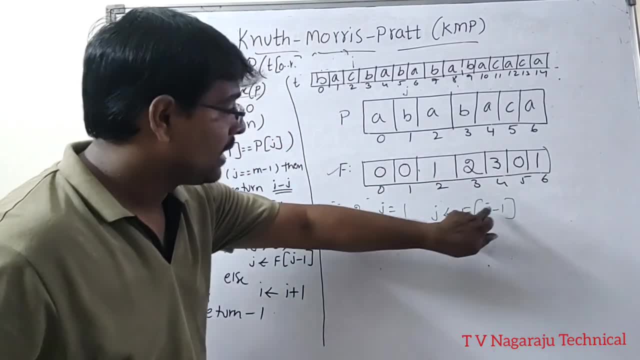 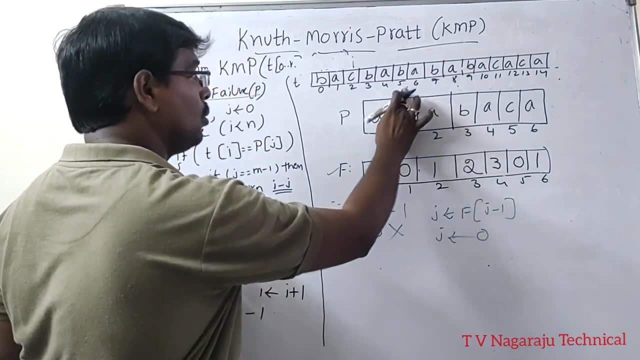 Now j is updated with f of j minus 1. j is updated with f of j minus 1. J is 1.. F of J minus 1 means F of 1 minus 1, 0. Now J value is equal to 0.. Whenever there is a 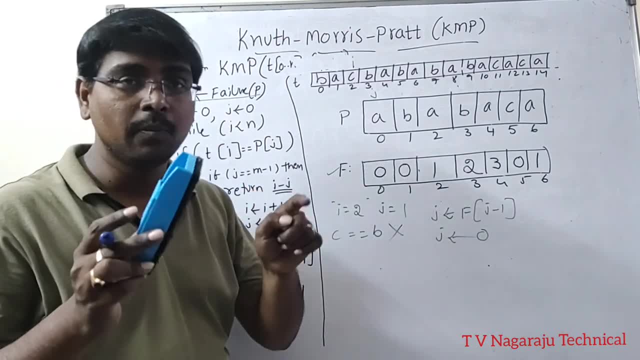 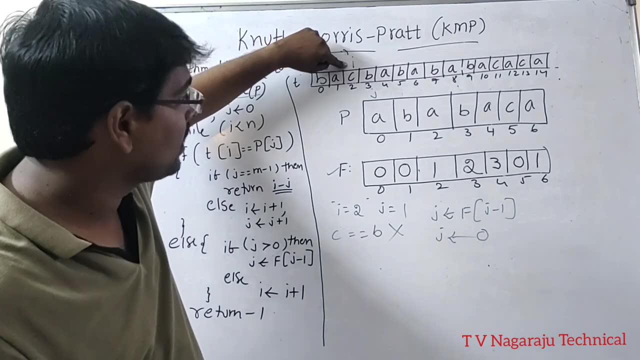 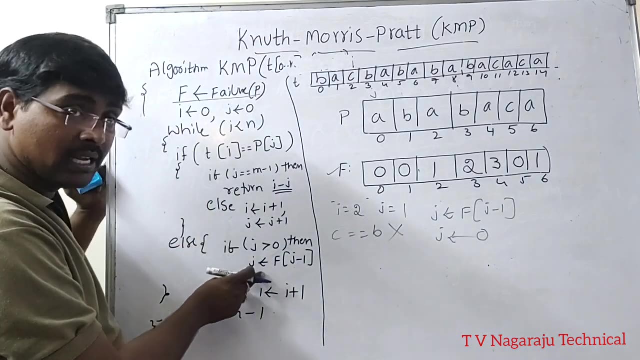 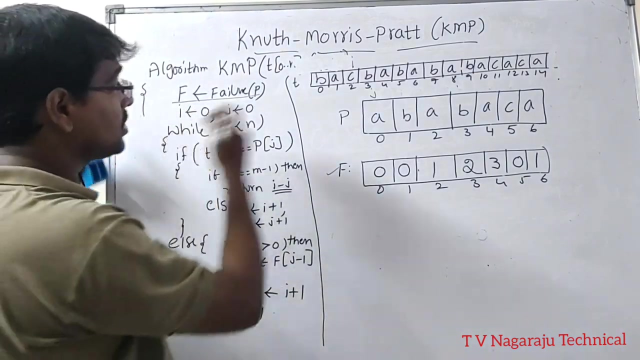 mismatch, use the LPS table. Simple purpose is avoid the backtracking of I. To avoid the backtracking of I, J is moved, J is moved. Okay, Now in the next iteration, is any I is updated? No, I is not updated. Else, this is completed Again, next iteration In the next iteration. 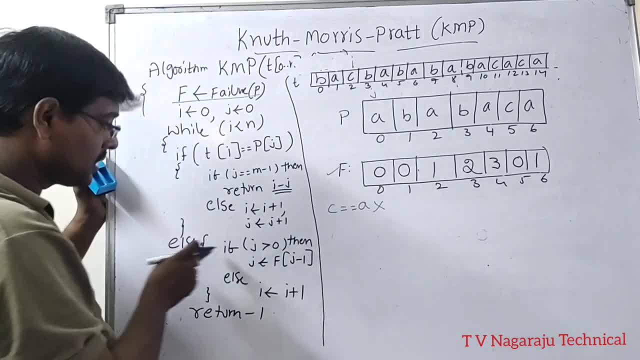 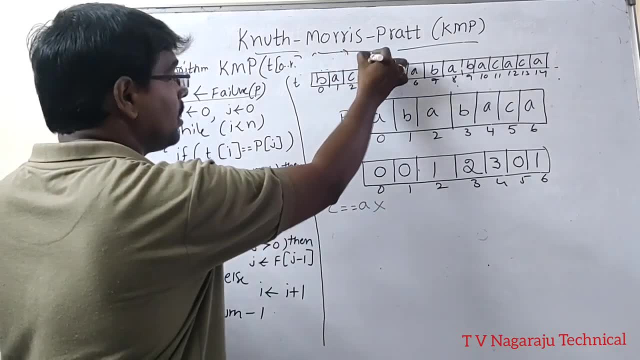 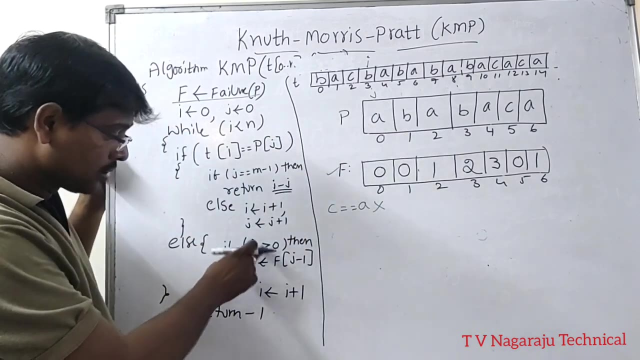 C is equal to equal to A- Condition: false. And if J greater than 0, false directly. else I is incremented by 1.. Now, this is I value. Next, iteration: B: equal to equal to A- false. This is also false Directly. I is incremented by 1.. 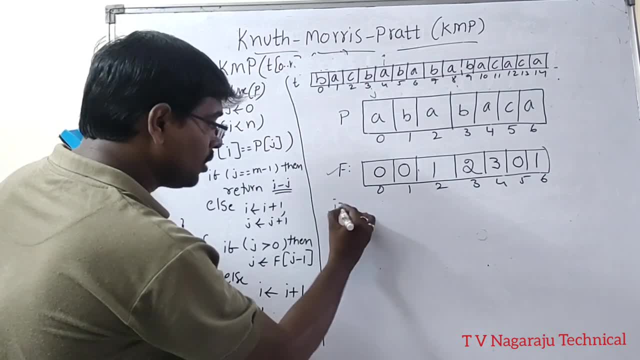 This is I value. Next, iteration B: equal to equal to A- false. This is also false Directly. I is incremented by 1.. This is I value. Right now, I value is equal to 4.. Yes or no? Right now, J is equal to 0.. Again, compare A equal to. 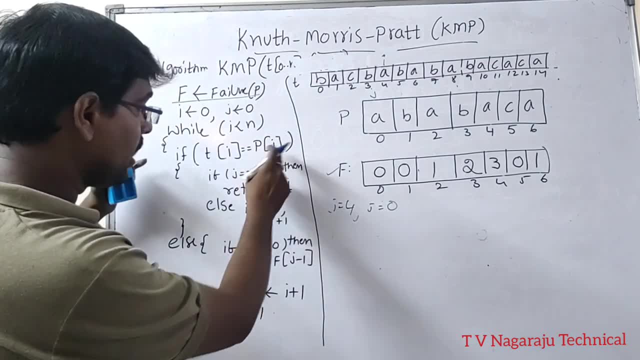 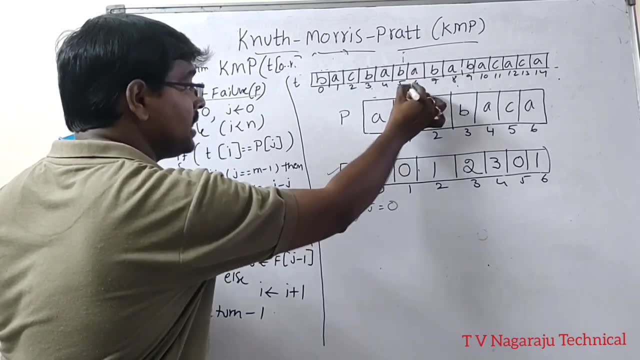 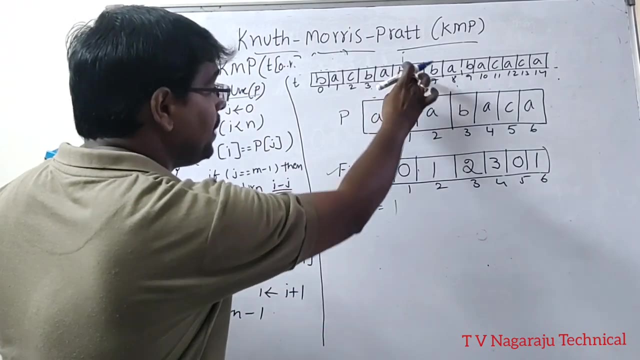 equal to A true A equal to A equal to true. This, if false: Yes, I is incremented by 1.. J is incremented by 1.. That is, I is equal to 5.. J is equal to 1.. Compare: B is equal to equal to B. Yes. 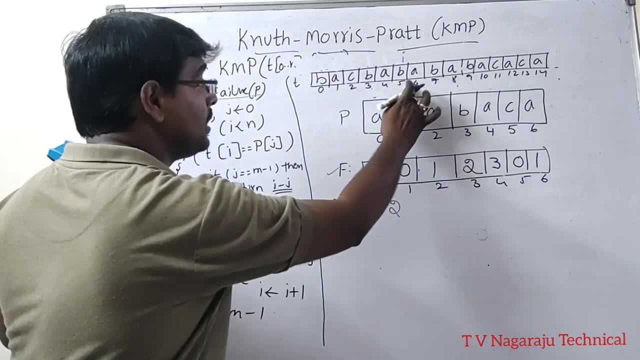 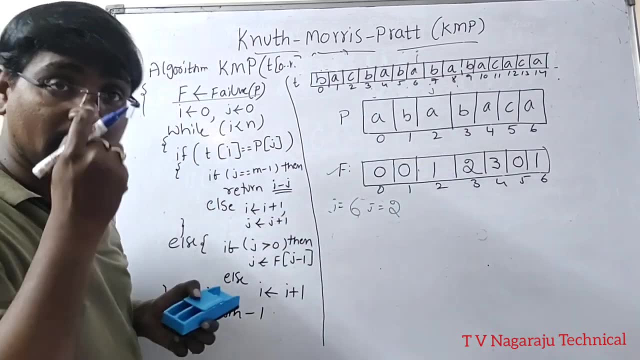 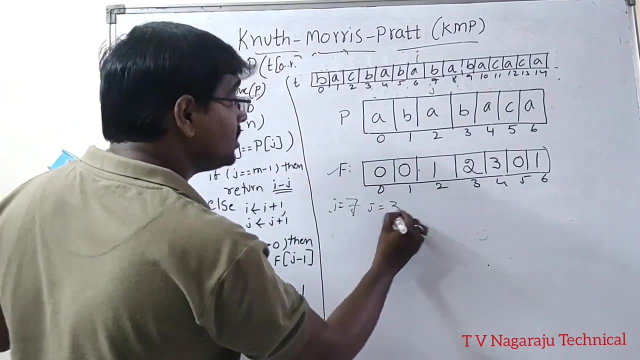 Again, right, I is incremented by 1.. J is incremented by 1.. Now A is equal to equal to A. Again, there is a match: A is equal to equal to A. So I value 7.. J value 3. Move. This is J value. 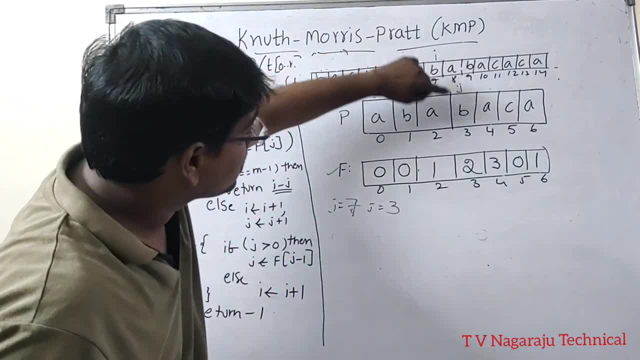 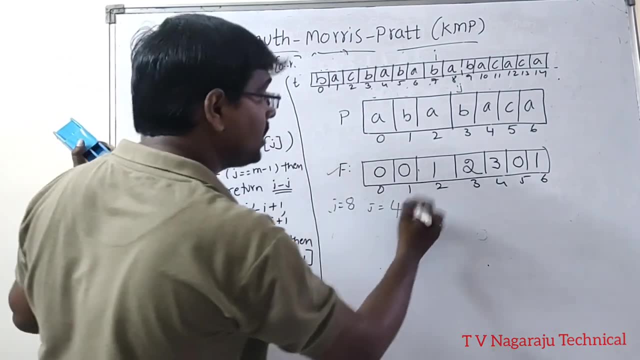 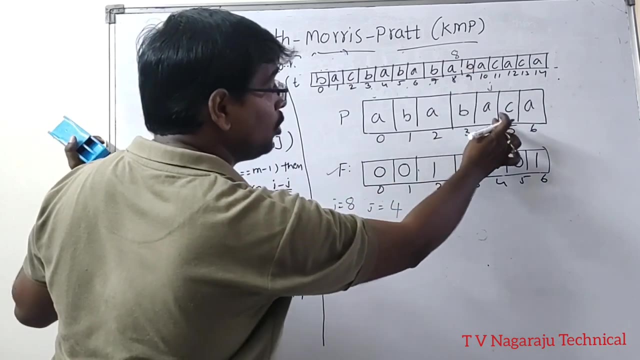 This is I value. Next, B is equal to equal to B. Again, there is a match. Again there is a match. I is equal to 8.. J is equal to 4.. Okay Now A equal to equal to A- Again there is a match. 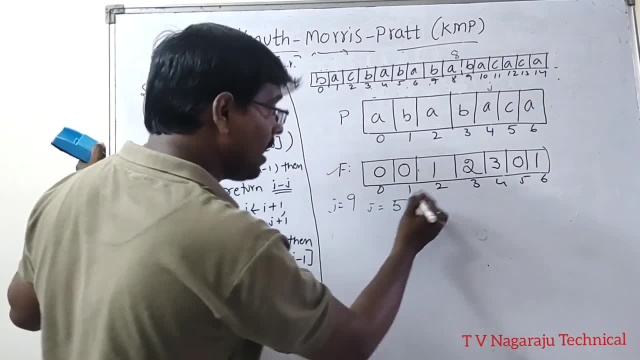 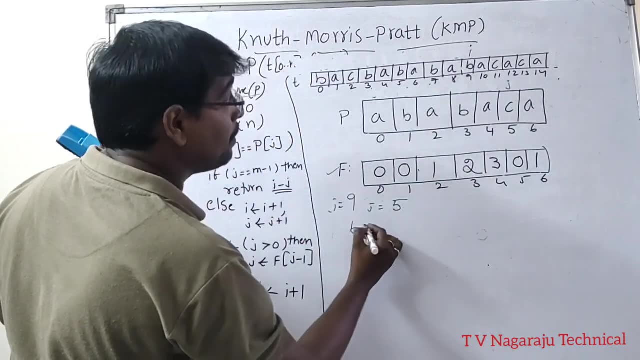 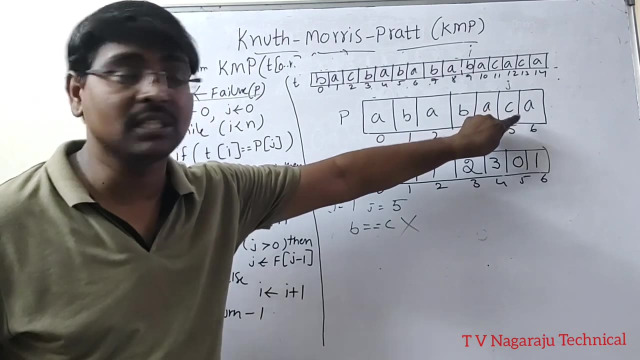 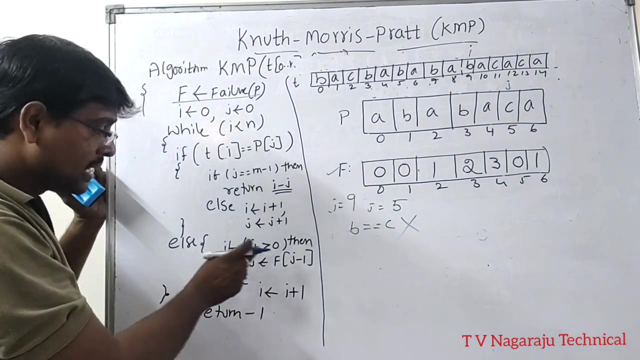 Now I value becomes 9.. J value becomes 5.. This is J value and this is I value. Now, B equal to equal to C. Up to 5 letters are matched. The 6th character mismatch B equal to equal to C. The condition fail. Move to else In the else check J greater than 0 or not. 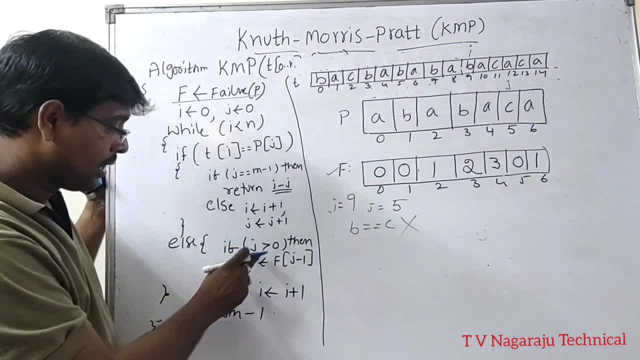 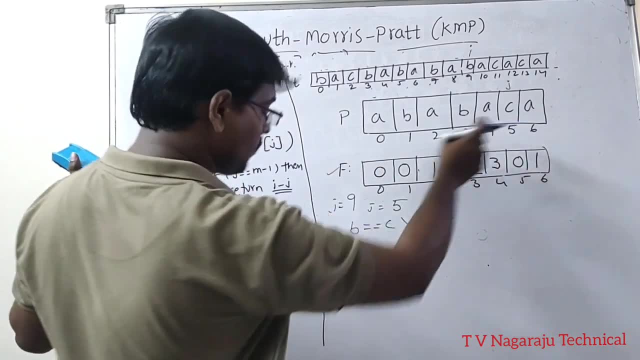 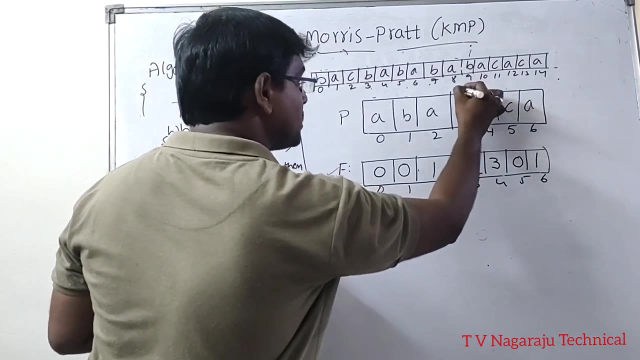 Yes, J value is greater than 0.. If what happened Immediately? J is equal to F of J value is 5.. F of 4. What is F of 4?? 3. Now, J points to this one. You got it. J points to. 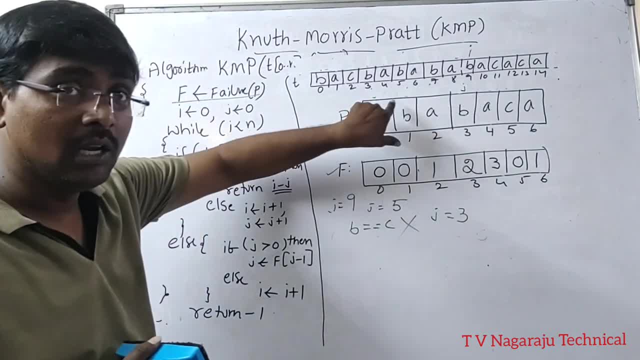 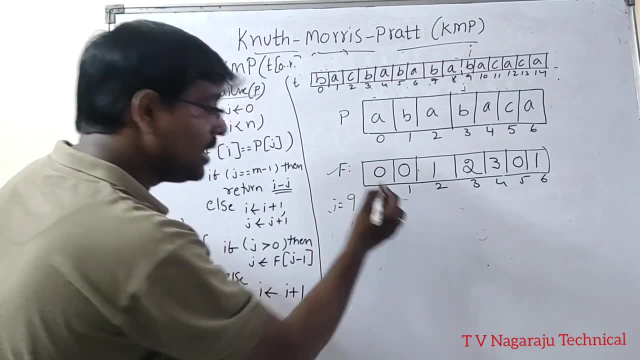 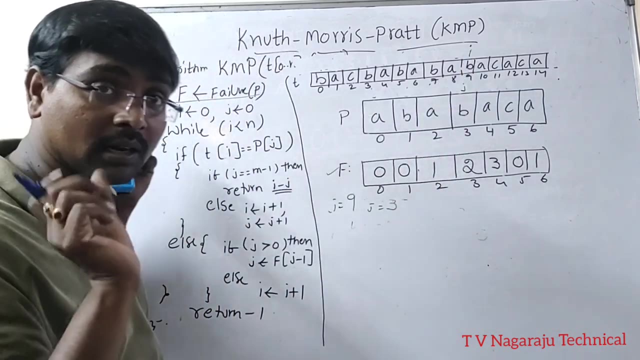 F of J minus 1.. Whenever J only move means I is not updated. Now what is the value of I 9? only J is 3.. Again, do the comparison? B is equal to equal to B. I think you got the point. 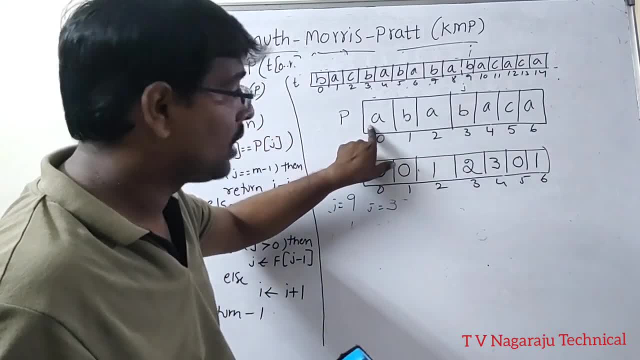 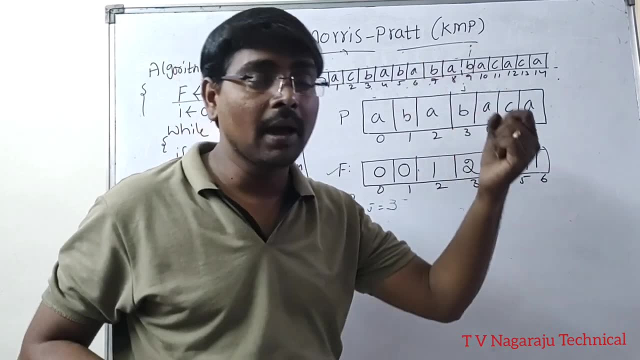 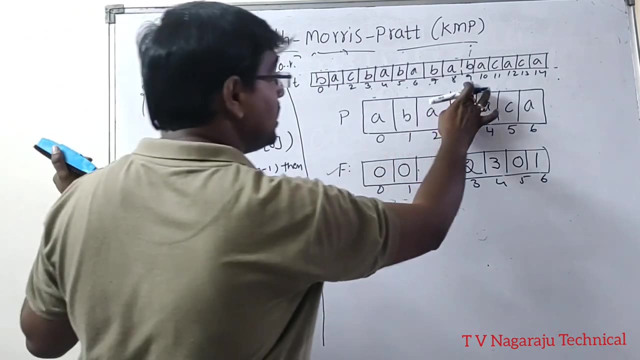 here, Instead of starting from the first onwards, once the element involved in the comparison in the next two times the already comparison elements are out. I did. That is my concept. B is equal to equal to BS. There is a match: J is incremented J value. 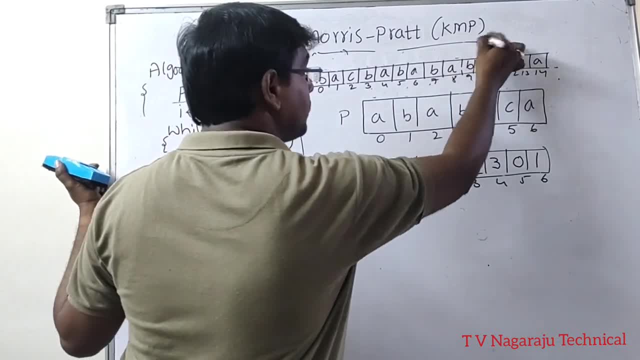 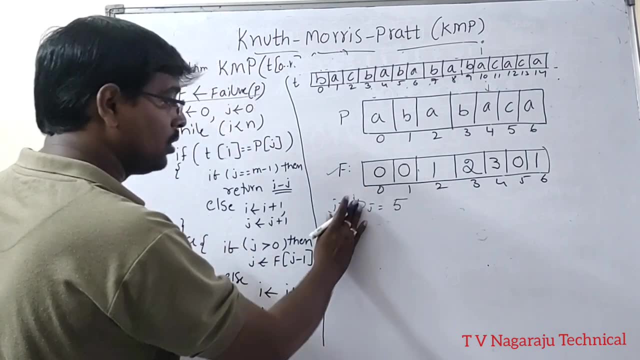 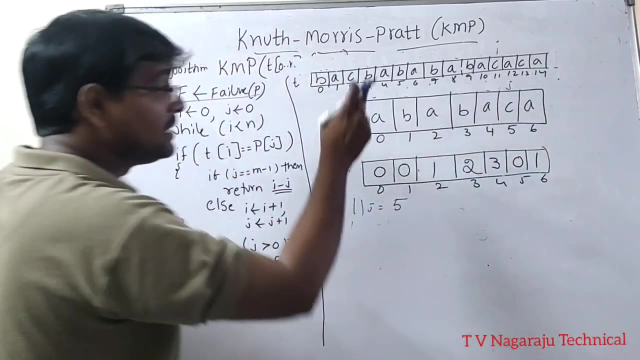 becomes 4.. I value becomes 10.. Now A is equal to equal to AS, A value is equal to equal to A. J is incremented. Now this is J, Now this is I. C is equal to equal to C. Yes, Now I becomes 12..